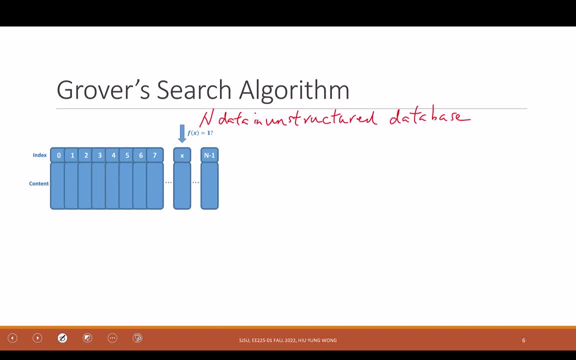 hey, are you Hugh? hey, no, are you Hugh? I will just do it one by one, keep asking, oh, is your student id this? and eventually, that's true, yeah, I am. then I find that student. this is like unstructured, right. if it's structured, maybe all the engineering students are in the engineer building. 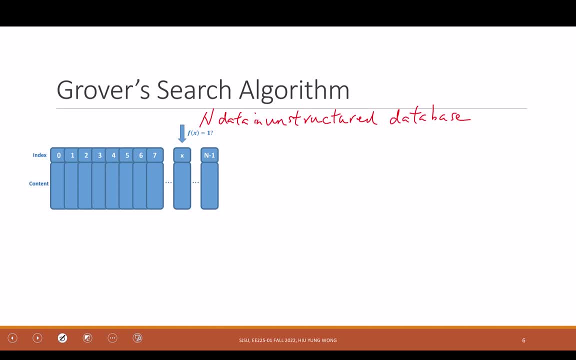 then I know that I'm going to find Hugh, who is engineer student. just go to engineering building, then the time of finding this data is much faster. so for this unstructured data I might. maybe this one is what I want to find. I will ask a question. I use something right or it can be. 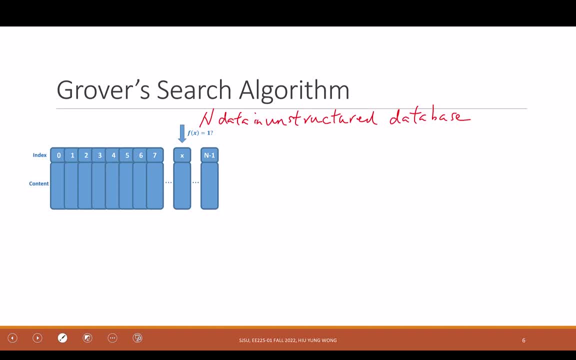 an image. I need to compare the image, which is a very expensive calculation. for example, what is the average time, I will find the data I want. what is the average time? right? basically, I am going to search right. if f, if x equal to a, I will get one. if x not equal to a, 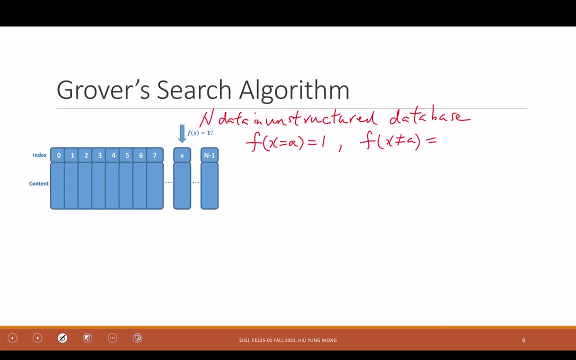 right. this x can be an index or just the data itself, but they are equivalent, right? I don't explain too much, but basically you do a computation. is that f, x, whether x equal to a or not? right, like my question? are you Hugh, right? and then no, I am not. then I find another student. 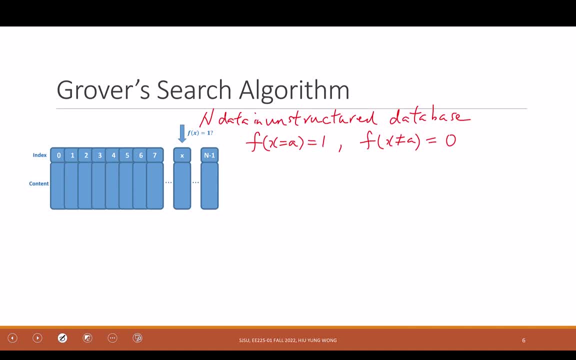 keep asking what is the average time I need to find the student. if I have n students say again n by 2, y because it's half, because is it really random, right, if I'm saying: i'm super lucky, I picked the right person? what's your name? oh, I'm Hugh. yeah, so I only need one. 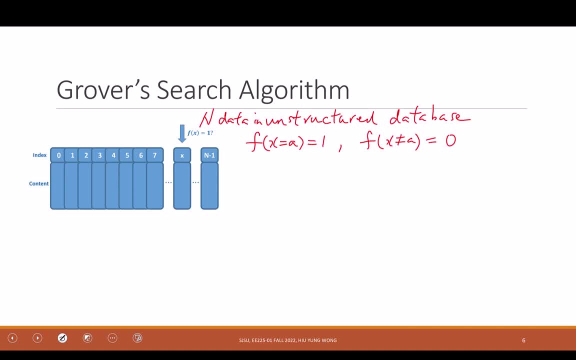 search if I'm super unlucky. I asked all the students and only to find the student I want the last one right. that is n right or in between. so on average, like a classical computer, it takes n by two. okay, naorama獸. What does it mean? I have 10 students On FH. I spent 5. 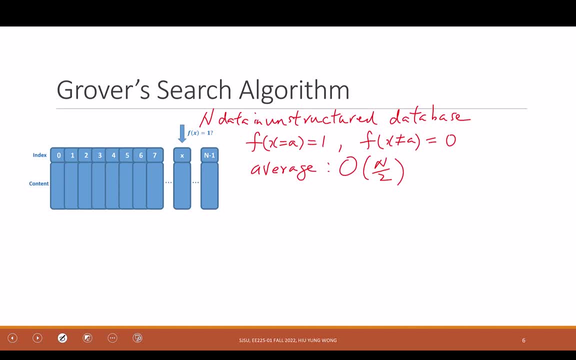 curies. I have 100 students, I spent 50.. I have 1 million students, I spent 500,000 curies. Okay, This is classical. But with quantum computing, which is the so-called group-first algorithm, it is. 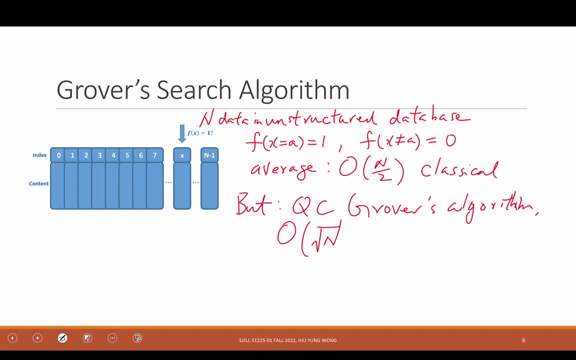 order of square root n. Okay, So again, what is the mean? And more precisely, if you want to know the exact number, it's pi over 4 square root n, And you will be able to prove this after you learn this algorithm. Okay. 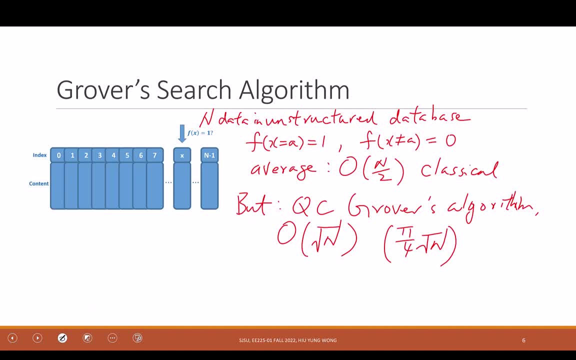 So just again, what does it mean? Right, If I have n equals to 1, the classical will spend 1 unit of time to search Quantum computing. also, you spend 1 unit of time Not useful. Spend so much money. Just no speed up. 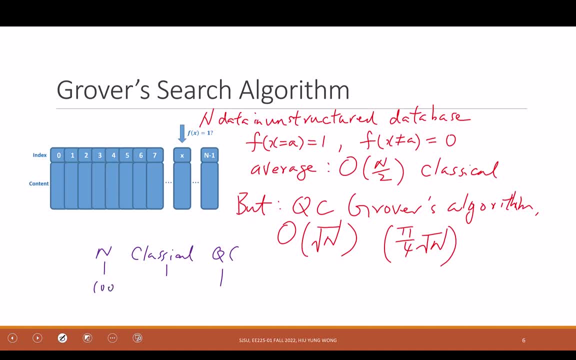 But if I have 100 students, the classical one spends 50 on FH And this one is spending 10.. Right, But now I'm going to remove the 2, because I really don't care about the scaling. as I said before, 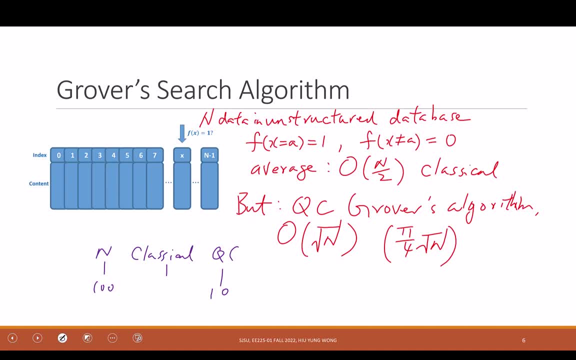 Right, Whether it's 1 million or 500,000, it's the same to me Too long. And if I have 10 to the power 6 students, I need to search classically. I need to search in the order of 10 to the power 6, 1 million times. 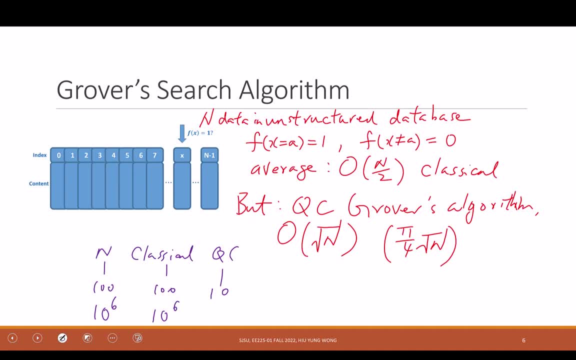 Classically, how much time do I need? I mean quantum computingly, 10 to the power 3.. Still a bit speed up, Right, I can do it now in half hours instead of 1 million seconds. Yeah, Why do I remove the 2?? 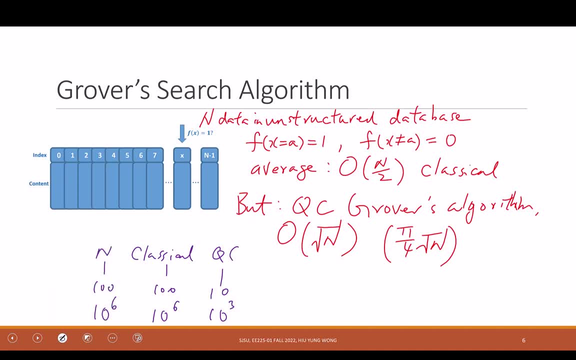 Because we really don't care about the coefficient, It's the n, what is really important in terms of the impact, Right. So this is just like order of n, Because the thing about this right It's If I tell you that I have 1 billion dollars. 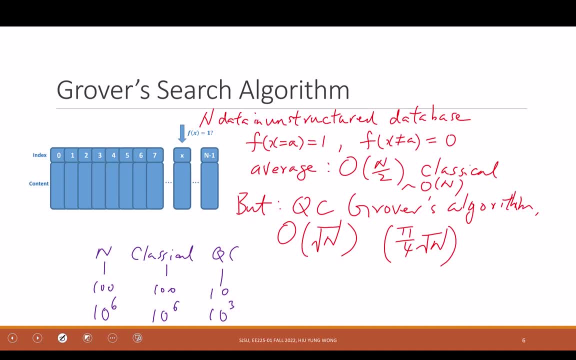 And you come to me and say, oh, you're lying. you actually only have 1 billion divided by 2.. I would still be very proud, Right? I'm still very rich For small. then we think about this: Do we care for a small problem? 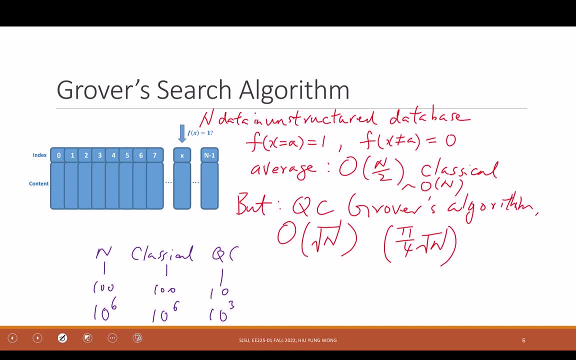 We really don't care about a small problem because we can compute it fast, While we spend time to analyze the complexity. Right, So we really care. It's a large problem, Right, So we really care, It's a large problem, Right. 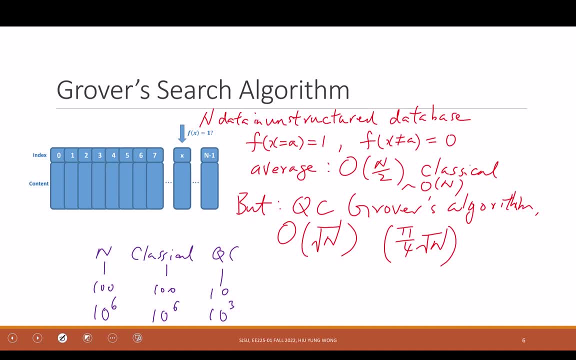 Today I have so much data. Tomorrow I'm going to have 1 trillion times more data. Which algorithm can help me to handle That? is not really n or n divided by 2.. Right n divided by 2 is not going to help my stock to go up. 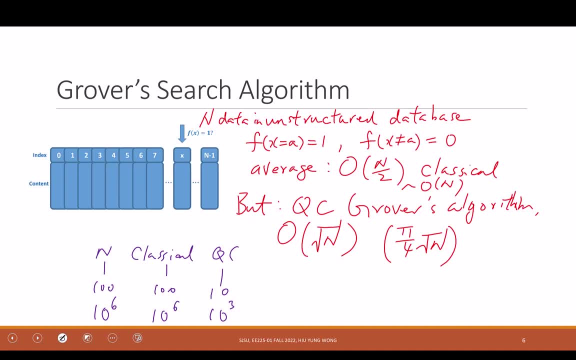 Right, By inventing an algorithm that is not n, Then that is a true breakthrough, And that's why this n divided by 2 is not really a big deal, And so we make it simple. But when you come to real implementation and comparison, 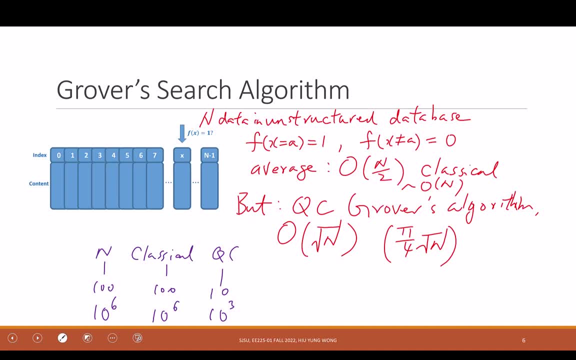 when they're close. yes, you might want to discuss this n But when you take this divided by 2 into account, then you need to go to even more detail. How about the preparation of the data? How about the power consumption for processing those data? 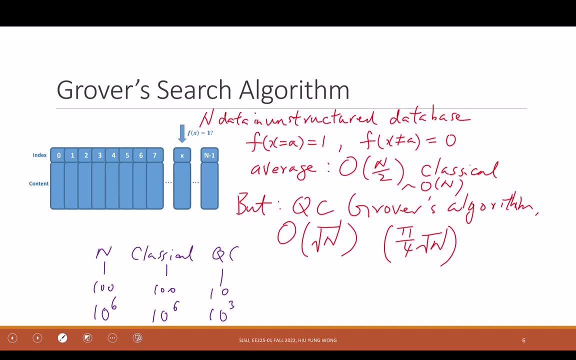 Right, Because this is only equates by 2 times, But maybe your preparation have a super big overhead, Right? So now we only look at a very coarse range. Okay, Yeah, But what you think makes sense, Right? But now we only care about large data. 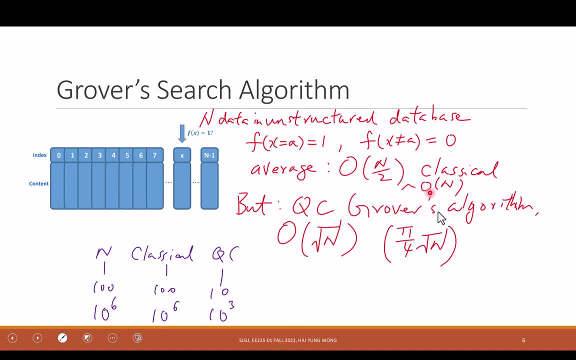 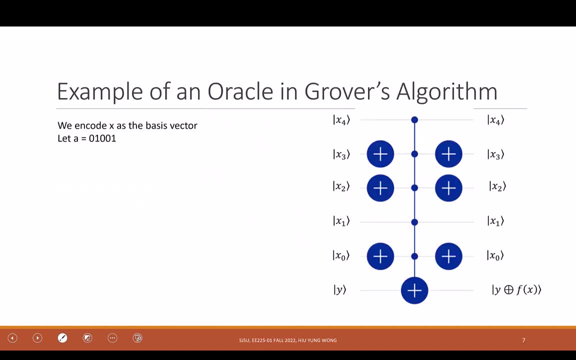 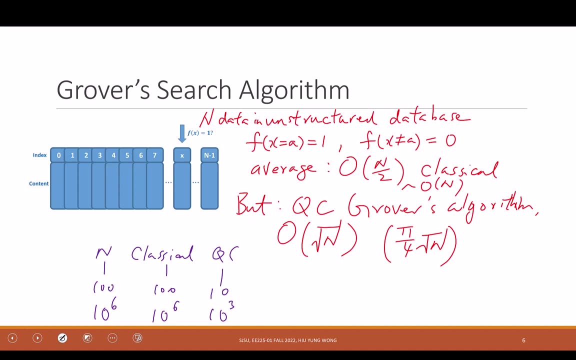 That's why we only need to talk about n instead of n divided by 2.. Okay, Good point. Okay, So we want to search the data. The goal is to search where the data is, So we need to keep doing computation. 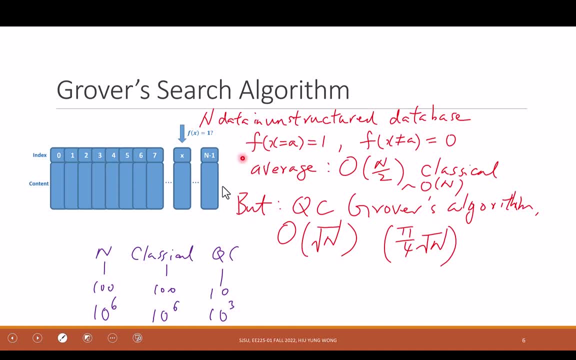 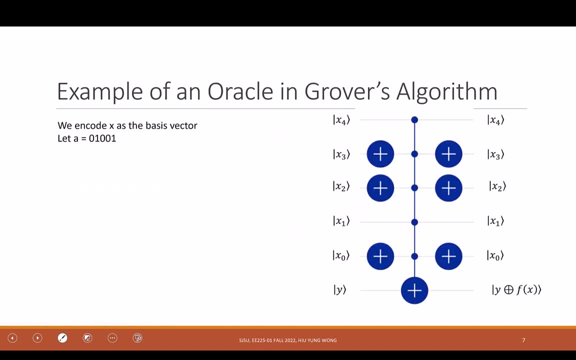 And the computation is to find out f of the index, f of 1 all the way to whatever. Now then, how do we do it in quantum computing? x is what we are searching for. So here come to the encoding problem. How do you encode the information into the quantum computing problem? 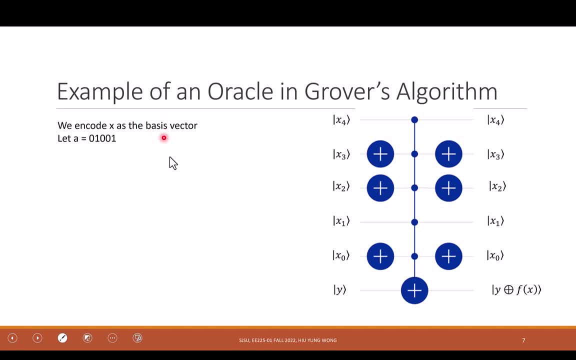 There are many ways. One of them is called basis encoding, So you store your information as the basis state. Okay, So if x, for example, what it means is that now I will formulate the problem so that each basis state represents the something that I want to search. 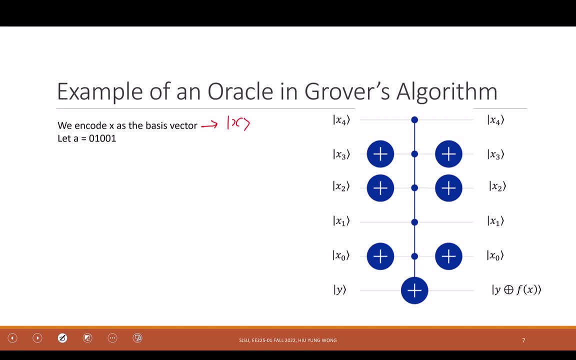 The index Right. So if I'm looking for, this can be student ID Right, Just like what I'm talking about, Right? Of course, student ID is equal to easy to do, why we need quantum computing, But maybe this is image mapping. 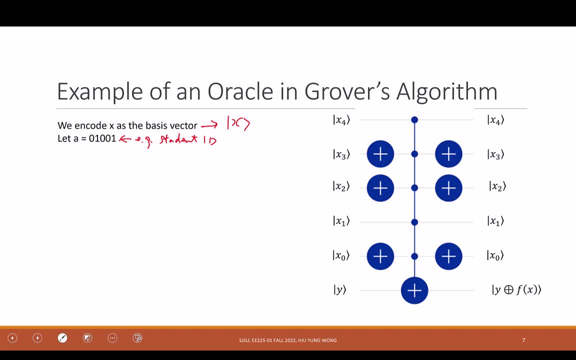 The image is super big. Right Info: you use a neural network that can save the time. My student ID is 01001.. And I need to search the record 01001.. Right, And yours is 1000.. So when I do the computation, 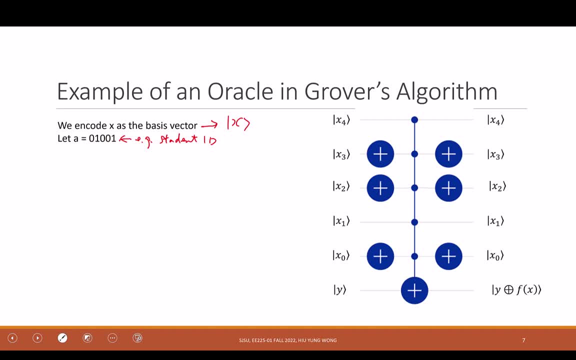 right in a classical computer. I'm going to find out what is f of a Right. I will try to compute. Take the x, Maybe. let me repeat what I said earlier. I look at each x. If x equal to a. 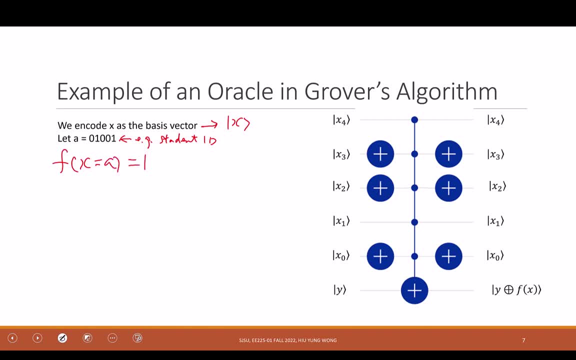 then return 1.. That is the function, Right. If f of x not equal to a, then I return 0. Right, So you see that my goal is to come up with a quantum oracle so that if the basis state is a, 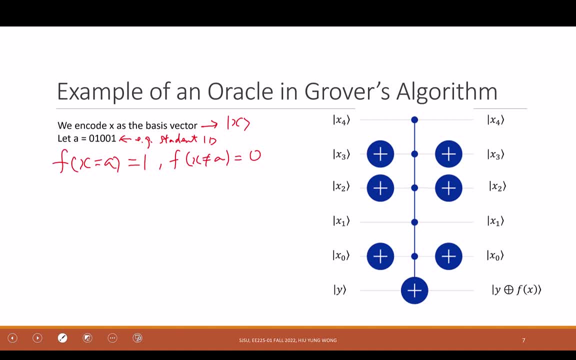 the output is 1.. If the basis state is not a, then the output is 0.. Right, This is just an example, And here I try to implement using a exclusive oracle. In the later session I will use I will use the. 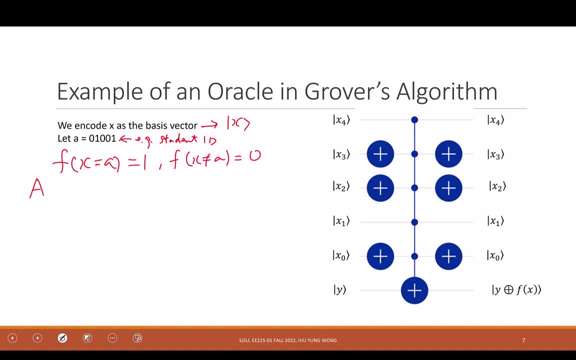 phase oracle. But here, just to give an example, since we just talked about oracle, I want to use this as an example, Right, So as an example, an oracle example. in this particular oracle, how can it help me to get? 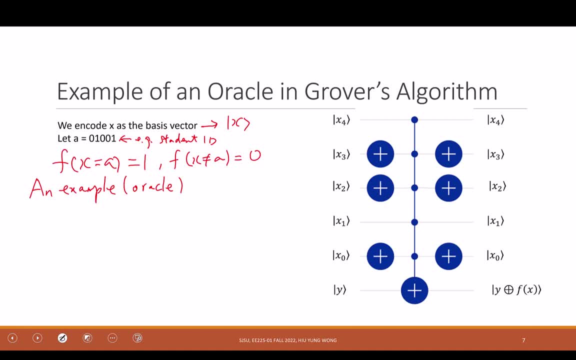 the a. First of all, how many bits do we have as the input? Right? Remember this box, Right? You just asked me what are the diagonal right. This is x. This is y. This is x. This is y, exclusive. 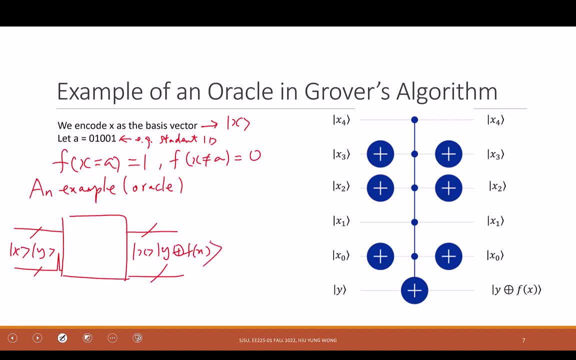 f of x. I want to implement this oracle. This oracle represents the problem I'm going to solve, which is to search for a Right. The problem I'm going to solve is to search for a, which means that you need to return 1. 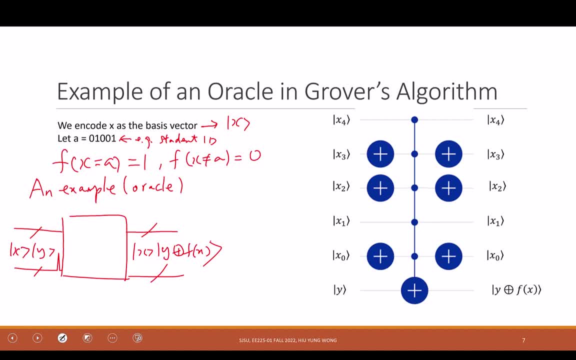 when it is f of x need to be 1. when it is x equal to a f of x equal to be 0. when it is not a Right, How many bits do I have for x? if I call this msb, How many qubits do I? 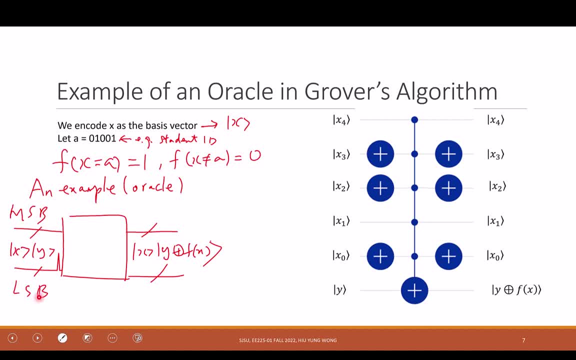 have for x, based on what I show you at the top, How many qubits are we using? 5. Right, 5 qubits, Because we encode it in the basis state, right? So you have 5 qubits. How many? 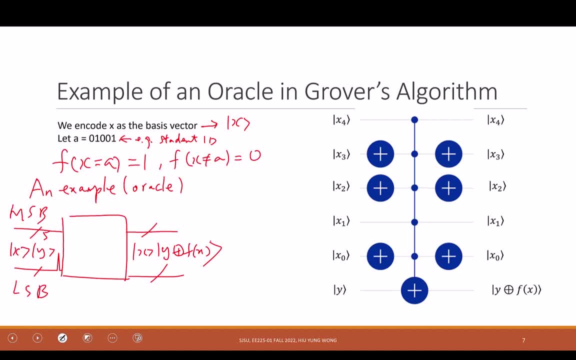 qubits do we have for y: 1. Because the output is either 0 or 1.. Right, So that's it. That's what I need to do, And now let me show you that why. on the right is a possible circuit: Right, So this is. 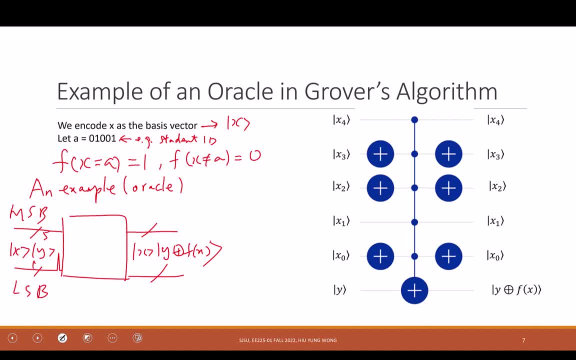 what you need to do in your homework and your project. Right, Not for Groover's algorithm, Right, But you need to create your own oracle. Now I want to tell you this is the correct oracle. Why? Because, if my input is, 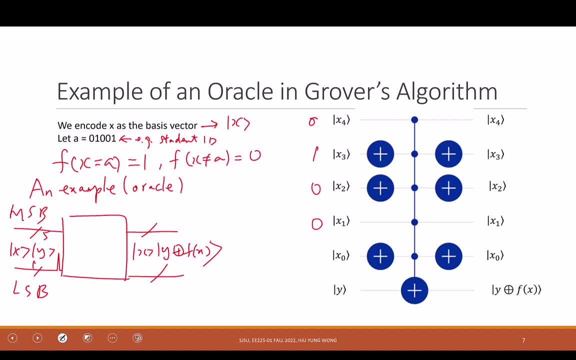 0 1 0 0 0. No, I have it upside down. What do you mean? No, My MSB is on the top. Do you see? I put x4?? Yeah, So in this case, I put MSB on top. 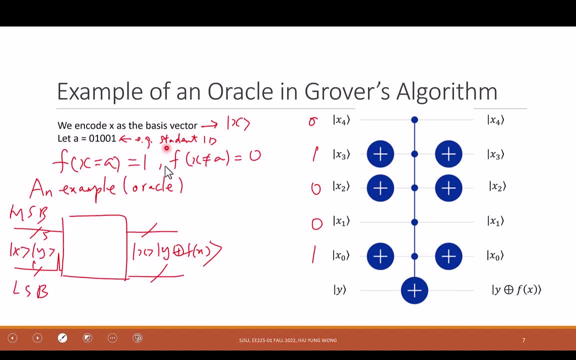 Not the IBM Q case, Right? So MSB is 0.. This is MSB, This is LSB. Yeah, So 0 1 0 0. Okay, But then I have the wrong circuit, Right. You want to say: 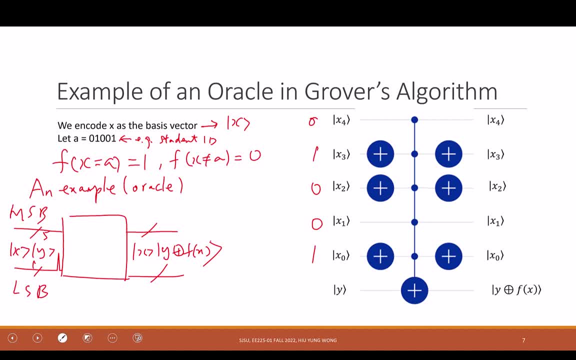 Yeah, I forgot to swap the circuit. Yeah, So this is wrong. Um, Okay, Yes, Thank you. Thank you, You are smart, Right? So, everyone, I made a mistake because I I was actually using LSB to draw this circuit. 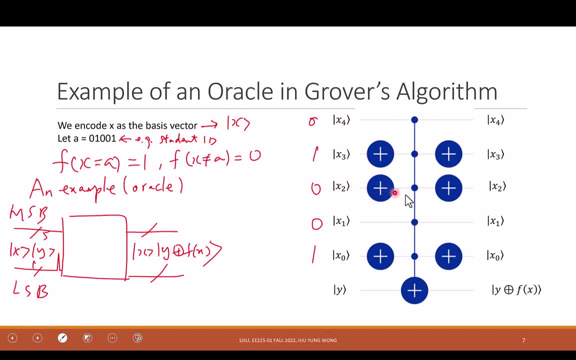 Right, But I already labeled them wrongly as MSB because, compared to last semester, I tried to swap it. I did not swap everything, So I'm going to change one thing. I know it's annoying, But he has a very good suggestion. 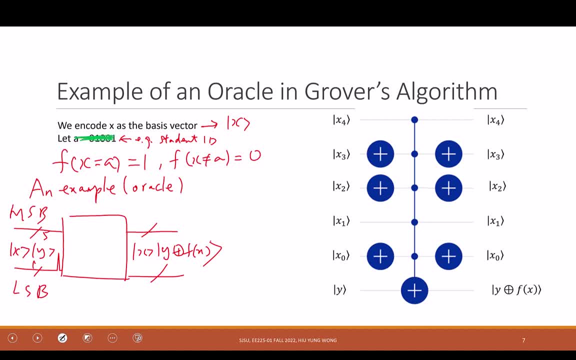 I'm going to change A. Okay, I'm going to change A to 1 0 0, 1 0.. Is that okay? I just think that I'm going to change it, Then everything is correct. Okay, So I start with 1. 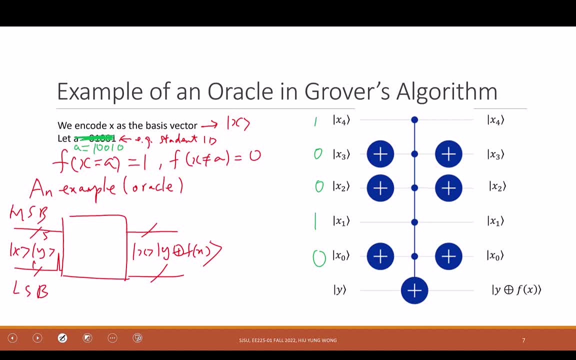 0, 0, 1, 0.. Is that? okay, That is the input. That is X, Right? What is Y? Usually we start with 0.. Okay, We start with 0.. After I go through the first set of gates: 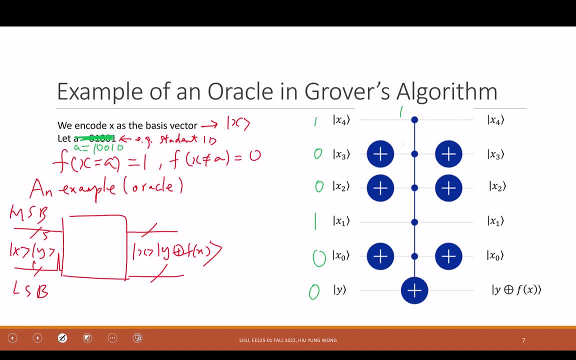 what is this? 1? What is the next one? X3? 1, 1, 1, 1, 0.. Right, What is this gate? Do you know? Can you give the full name? This is control, not gate. What is the full name of this one? 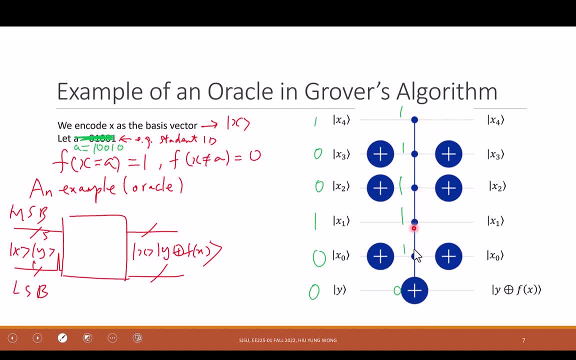 Control, control, control, control, control, not gate. Okay, Yes, Indeed, that is true, But what it means is what, By your definition, as you know before, this only happen if all of them are 1. Right, So if I really want to write this gate, 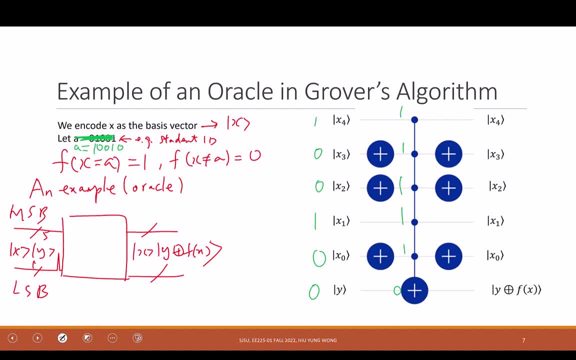 when I apply to a basis state. this is like I call it: C5, 0.. Right, And I apply to this one. I have X4, X3, X2, X1, X0, Y. This is a 6 qubit circuit. 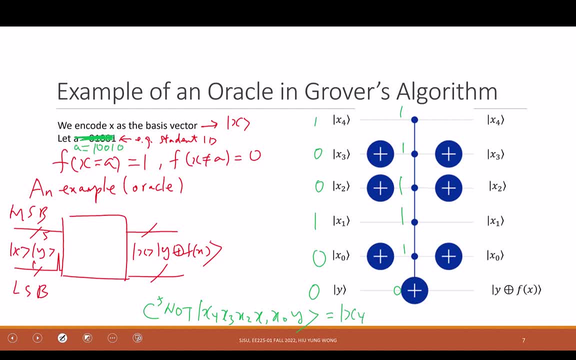 It is equal to X4, nothing change. X3, X2, X1, X0- Nothing change. I try to separate them, And then Okay, And then this one. I am going to do X4.. Do you remember how do you write the equation? 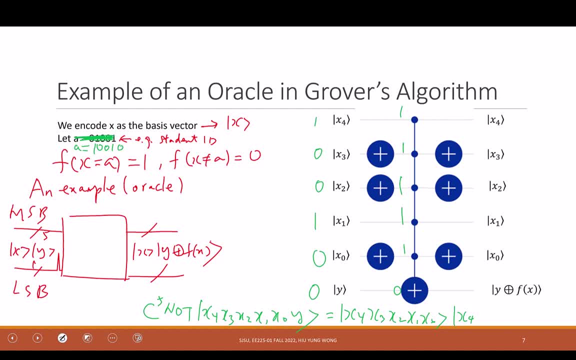 for not control. not, They all need to be. need to control. you use exclusive, all Right, But now you need all of them to be 1, first, Right, Right. This is talking about the basis state. If any of this is 0, don't. 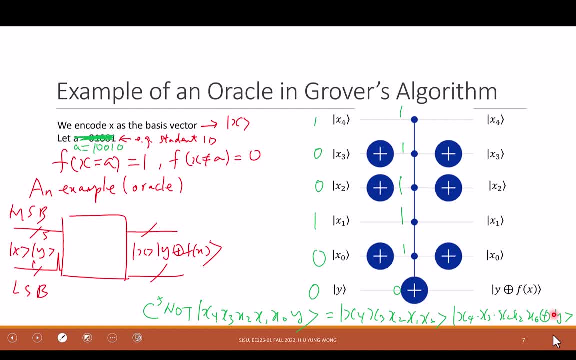 change Y. If this is 1, negate Y. That is meaning of the control, not Right, But just that we have. besides your parents, you still have your aunt or whatever. Keep controlling you, All of this Right Making decision whether you should get married to that boy. 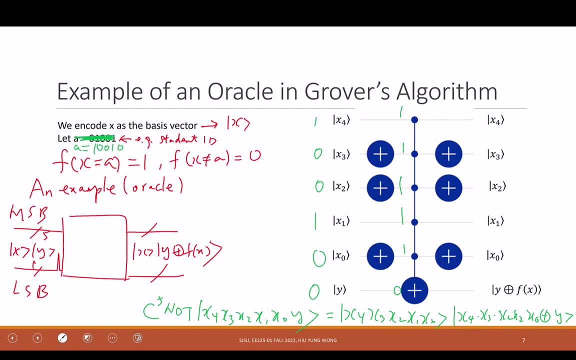 or that girl or not. Control, control, control, control. not Okay, Yeah, It can be changes. Yeah, Then you need to change the oracle, But that makes sense. No, no, It doesn't make sense here, Right, Need not speak up, But that. 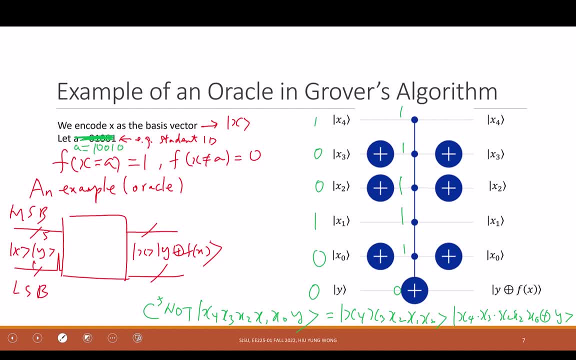 makes sense, because the oracle should contain the information of your problem, And your problem is FA equal to 1. And that's why you, your oracle must be different for different problem. I know it's useless now, But do you understand? I think that. 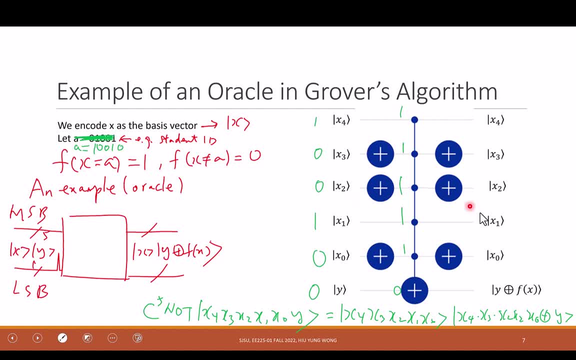 if your A is change, then the oracle needs to change, Because the problem of finding you in this class is different from the problem of finding me in this class, Because we have different student ID. You understand that right? Yes, Now practical, as I said last time. 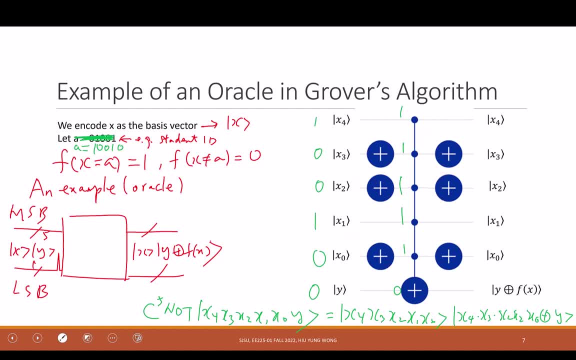 for oracle? you first of all. if you can construct this, for this simple one, you don't need to search Because you already know where it is Right. Remember: you only search one. Yeah, So you need to rely on some physical mechanism, Which I also don't. 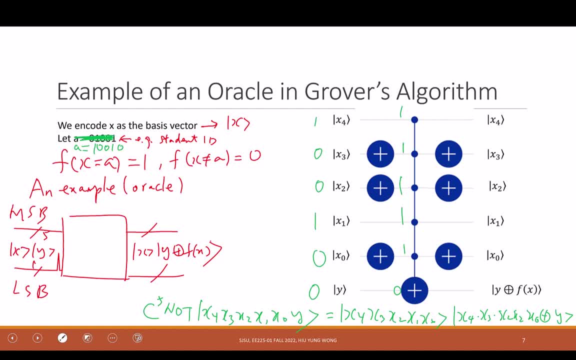 know exactly how to do it. You can decompose it right. There will be some algorithm that will help you to automatically build up the circuit for different oracle, For different A. This one is just a toy model example for you. It's not going to gain any. 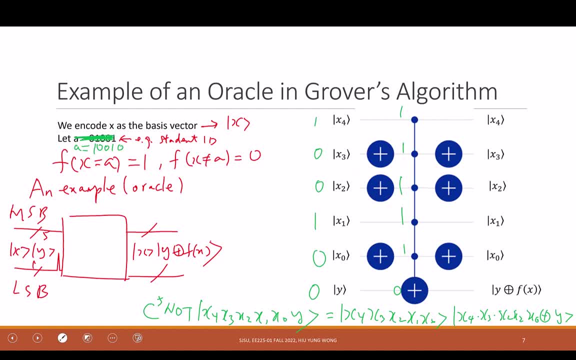 advantage, even if it works. But there will be an algorithm to help you to decompose. You say I'm searching for this, this number, and then you just come up with all the quantum gates that is necessary to implement that oracle. Or maybe there is a physical system. 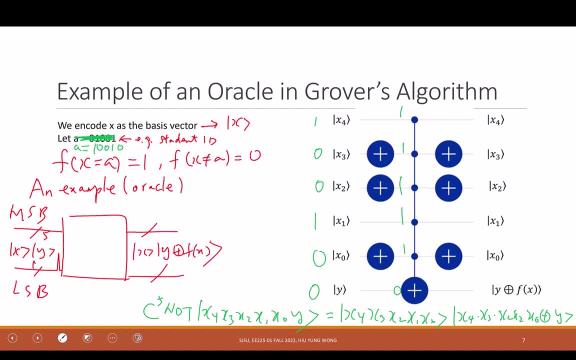 You don't know what is inside, but you know that it gives you something like this. So this is just an illustration of the idea. So that is a good question. I probably did not really answer well, but I think about that. Okay, Good, So then. 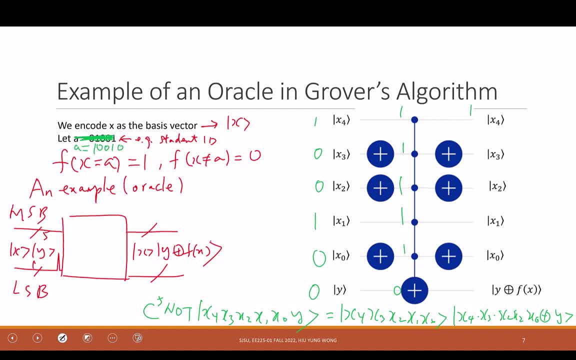 after the last gate is going to be what? 1 0 0, 1 0. So the important thing is: the x does not change, It's still the same, But the y equals to. indeed, y is 0, exclusive of if it is 1, right. 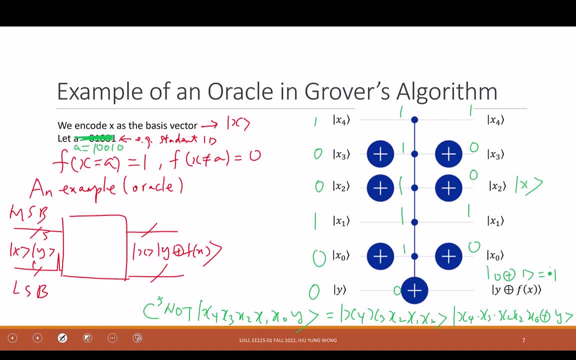 This one gives you 1 right. I mean, the answer we are expecting is y exclusive of f of x, but f of x is 1, now right, So I should get 1.. And indeed, what do I get? I get 1.. 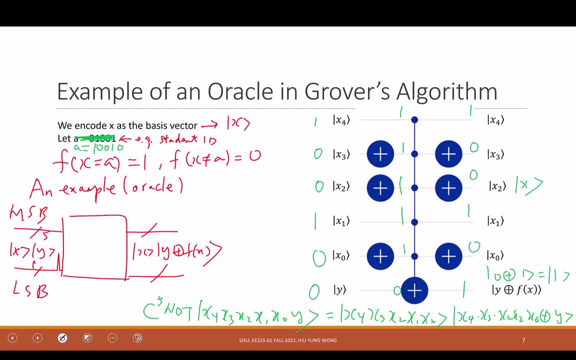 Right, Indeed, this is equal to this one. This circuit make the output equal to this one, right. So this implemented the oracle. They are just regular, not gate. Why do I need it? Because I want to rely on this control, control, control, control, not. 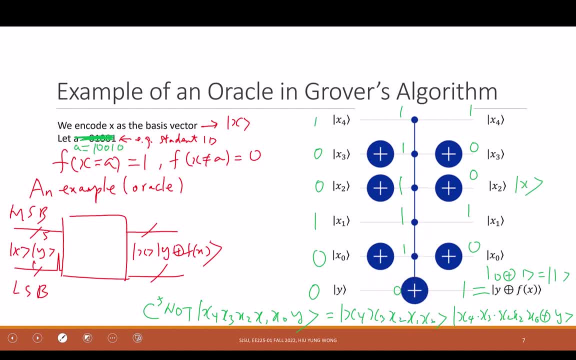 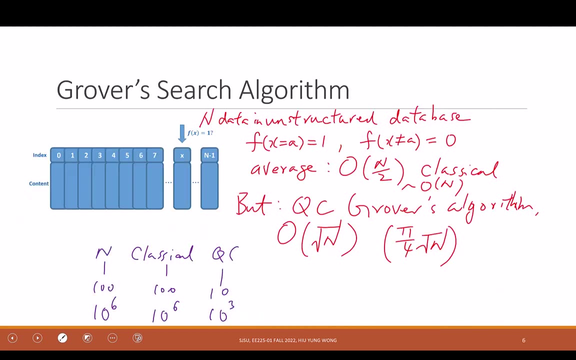 to Yeah, Yeah afterwards, but because by this oracle? why do I? we need this free, very good question. because we need to keep the x unchanged, based on exclusive oracle. Do you see that? That is the definition. x cannot change If you don't put back this. 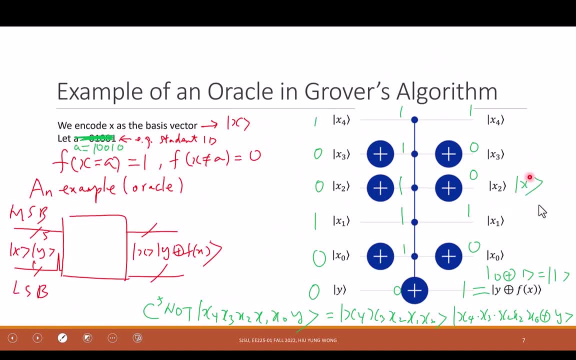 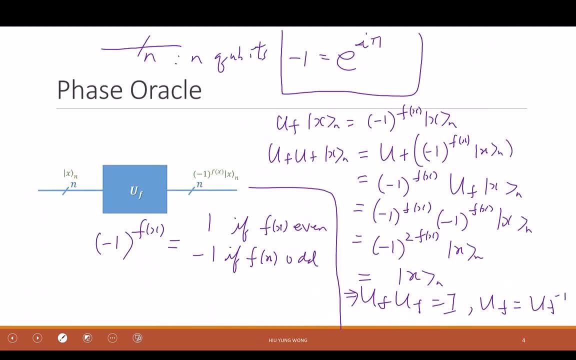 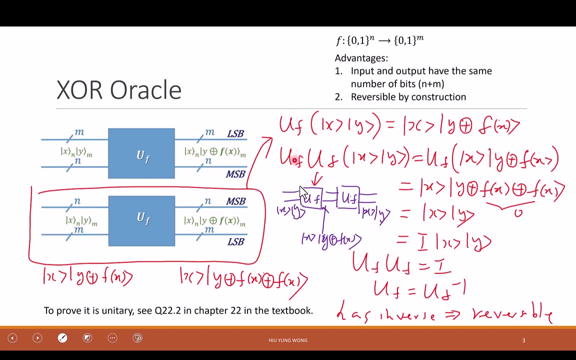 not gate. the output will be 1 1 1, 1 1.. It is no longer x. You rotate it. I care about that because this is yes, the information might come from y, but I care about that because that is how I get this. 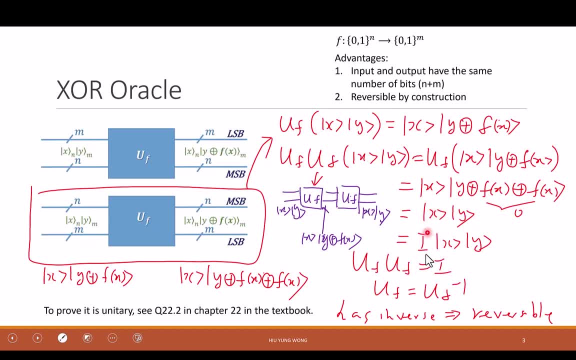 reversible. If this is not x, I cannot say this is i anymore. That is the definition, Right, this is the criteria you need to follow. yes, you can say maybe I only care the middle, but not really Think about the deutsch algorithm. What do you measure? You measure. 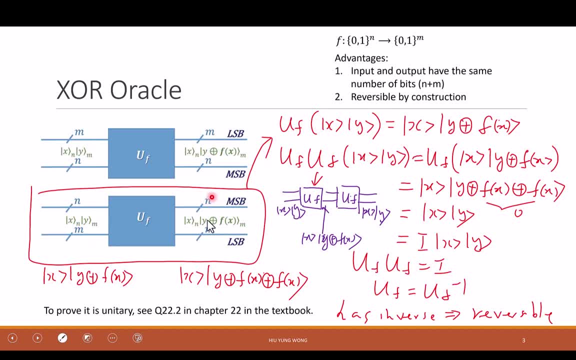 x. you don't measure the y, right, you measure the msb. actually, the bottom one are the one you are going to dump, although the bottom one contain the information, but because they as a whole, the whole system as a whole, contain the information. even you don't measure the bottom. 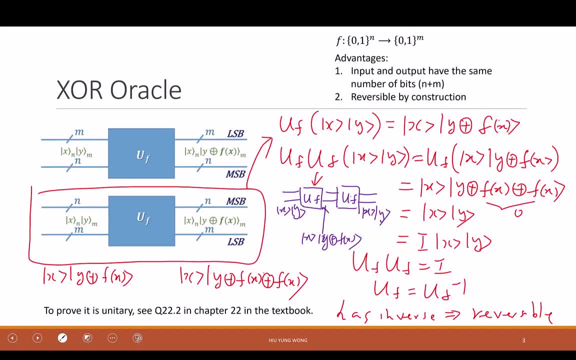 the information at the bottom affects the top. but that is just a simple one basis state, right, when you go to superposition, then you see the effect. do you remember? when you go to superposition, you do you measure the top one, what is left, the plus state or minus? 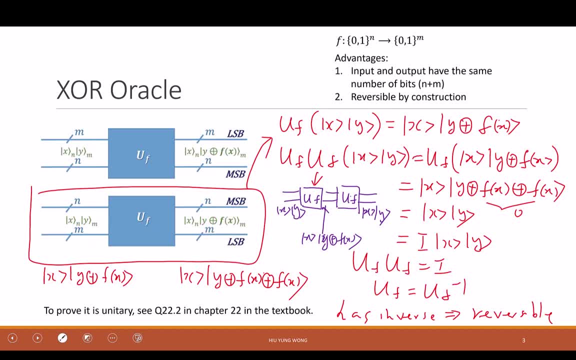 state is left really depends on what is at the bottom and the bottom got cancelled or not cancelled. depends on whether it is balanced or not balanced, right. so let's summarize what he said, why we need the top to be x when it comes out. that is why 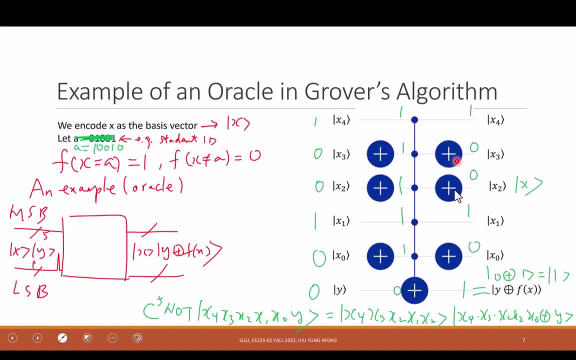 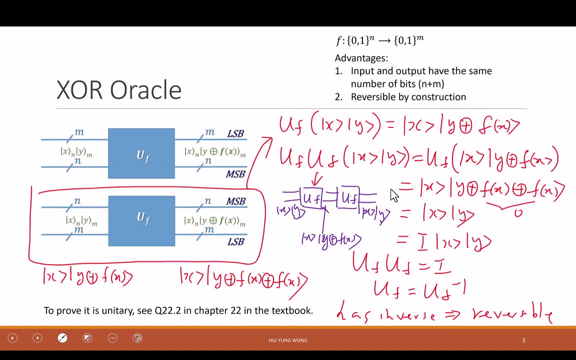 we still need to convert this one back to this not gate right. why we need to keep this as x? first of all, because we need this so that we can make sure this one is a reversible quantum gate. if you don't have this, if this x is changed to arbitrary, 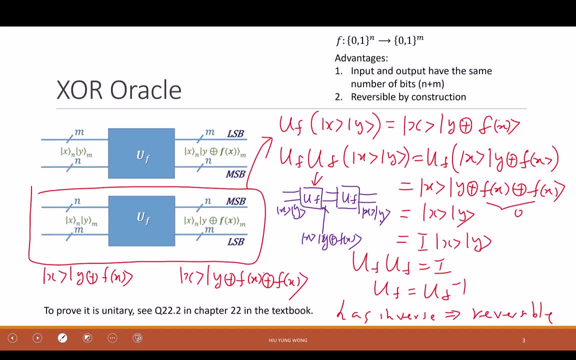 things, then this is not reversible. first of all, might not be reversible. right, our proof is based on this. is this: okay, no, but for quantum gate you want is using quantum mechanics. it needs to be reversible. yes, we don't go back, but then this one cannot be implemented physically. if 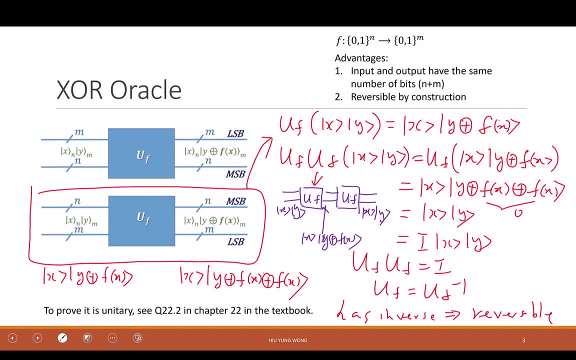 you cannot go back. remember why quantum gate needs to be reversible: because the quantum mechanics is reversible and if you have something not reversible it means you cannot implement by using physical quantum mechanics. it won't work. for example, you say: can i have a pulse shine to here so that it's not 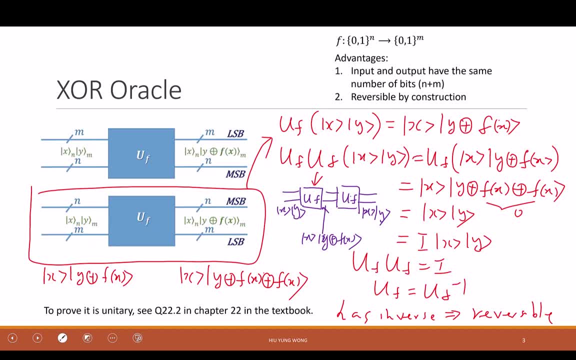 reversible? no, because quantum mechanics say that it must be reversible, so you cannot find such pulse. basically, it means that you cannot implement a gate of the type you are talking about. excuse that to you, that is right, but the nature say that you need to keep it. you can don't look at it. you. 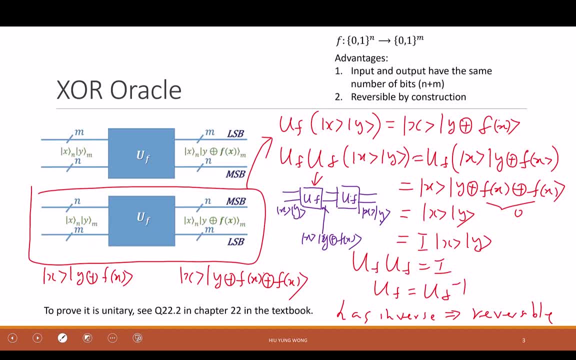 discard it as rubbish. but the nature is that it need to be exist, because if it doesn't exist, this is not a operation allowed by quantum mechanics. the quantum mechanics say that if you rotate this vector to this side, you should be able to rotate it back, and what you're saying is: 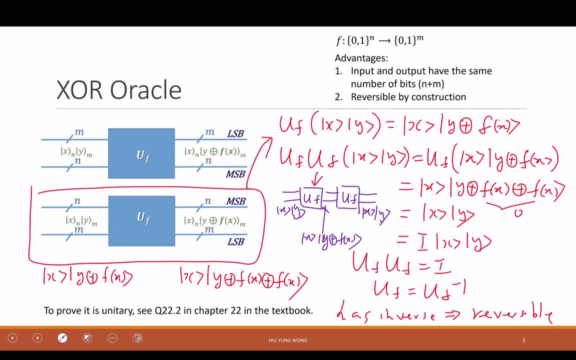 that it might not be able to rotate back and you won't be able to find such physics to implement this rotation if you cannot rotate it back. make sense or no? okay, maybe think about it right, but the main point is that this one must follow the physics. 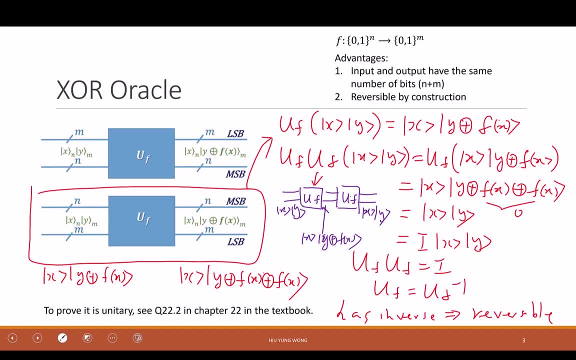 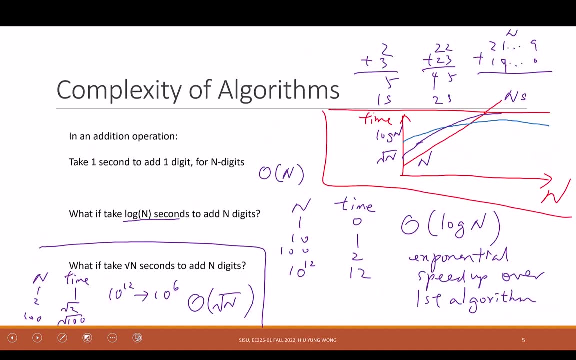 and the Schrodinger equation say that it must be time reversal. okay, you can go back. right, if you cannot go back, then it means you cannot find a physical way to do that. okay, that is the first point, right, and that separate point. he was saying that 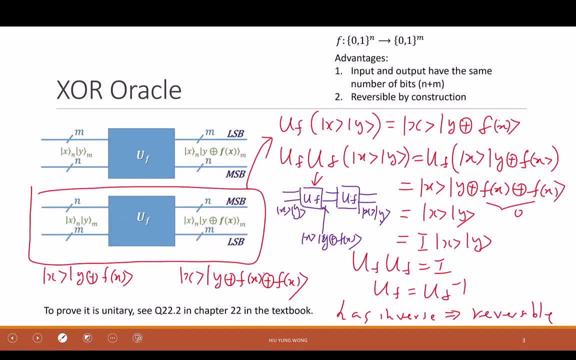 we only care about, maybe I mean the bottom- already contain the information. right, even you screw up- let's say, the nature allows us to do that. even you screw up the top. what is the problem? but no, this is a whole system. if you look at the deutsch algorithm. 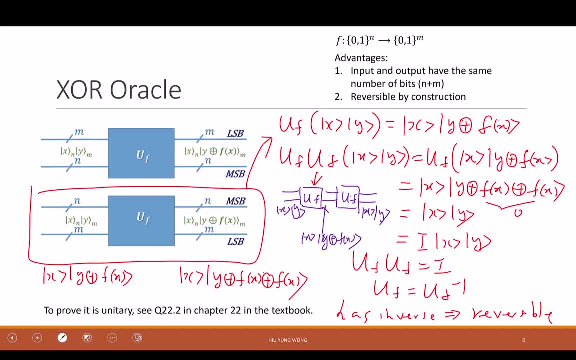 the way we get the answer is that we only measure the MSB and the MSB will tell us whether it is balanced or not, because the LSB will cancel themselves when it is balanced or non-balanced. so the effect is such that the reason you always get plus is because 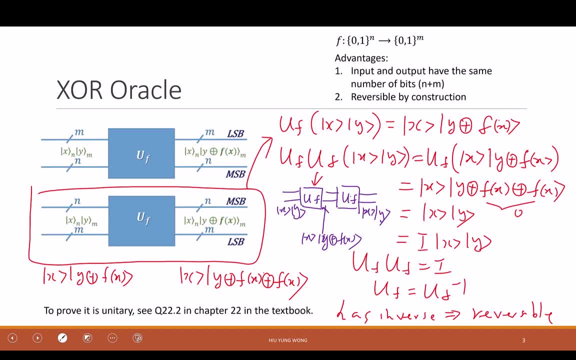 that function, make the MSB cancel. even you don't look at the MSB, but it has some effect to your measurement result- not inside out, after all, right. so this one is important. you try to think about that. just go back to the algorithm. go back to the deutsch algorithm. 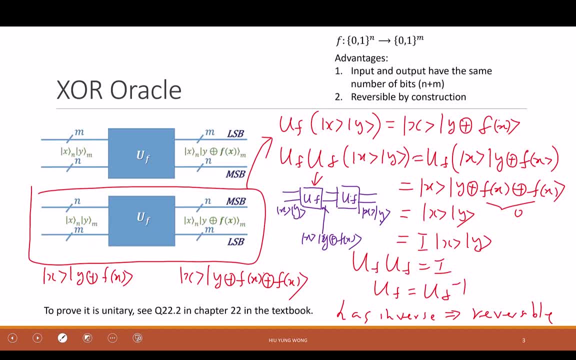 right. and then you tell yourself: now I just dump away the MSB, see if you can get the answer right. you and then probably you won't. and then you ask yourself then why I can get the answer. even the MSB does not contain f of x right. 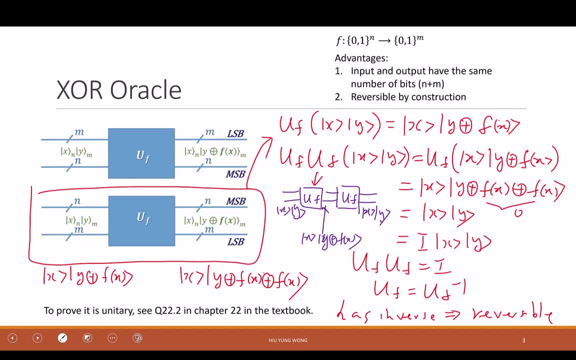 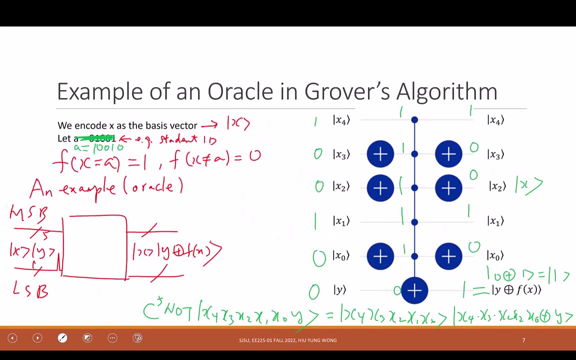 and you see that, because the LSB is doing some destructive or constructive interference that allow you to get the answer from MSB. that is the core. I say it, but you need to verify yourself, right? but that is a very good question, right? and that really tell you what to do with quantum. 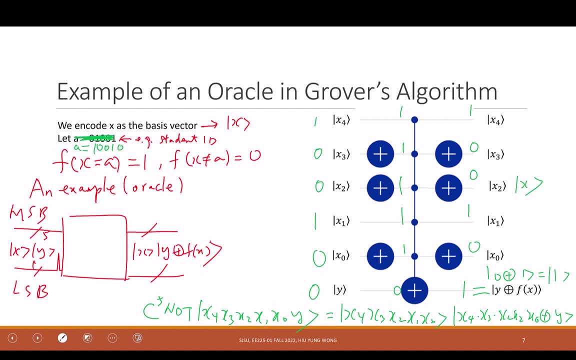 oracle and you should not make mistake now in the exam and you can try to add other things. I can quickly show, for example, if I do: this is a right. this is x, not equal to a. for example, let's say it is 0, 0, 0, 1, 0. 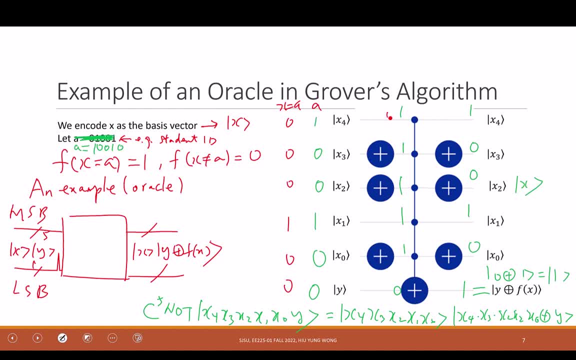 right, then if you go in, this is 0, ah, 1, 1, 1, 0, 0. right. second to last will be 1. sorry, yes, yeah, but then control, control, control. not one of them say no. unfortunately, probably the mother say no, you cannot. 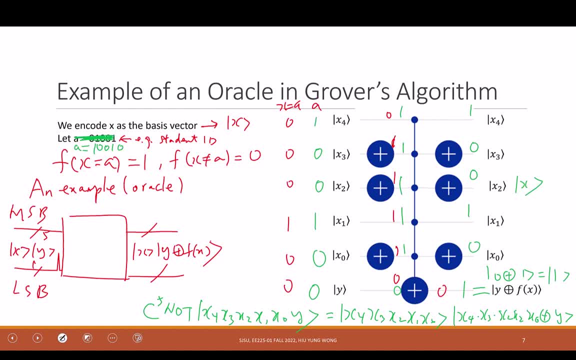 marry. then what? do you get 0 right, and do I get it right? yes, because f of x supposed to be 0 right. so 0 exclusive of 0 is 0. I do get 0 right. so that is a way to look into the quantum oracle. 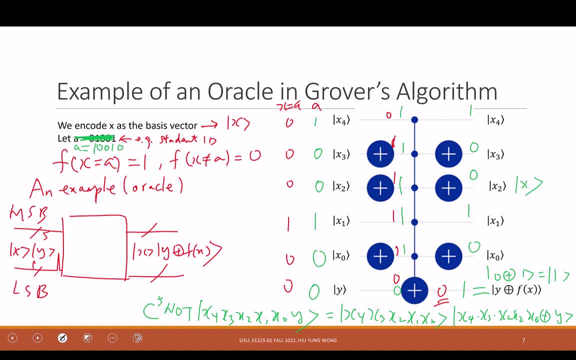 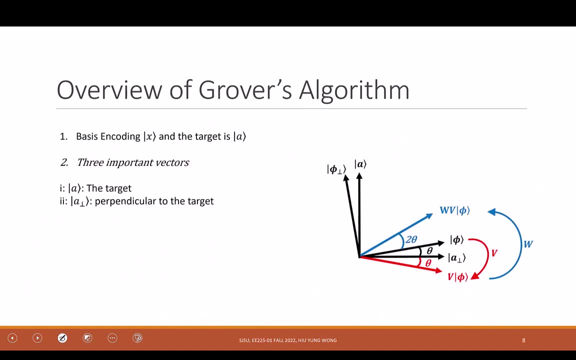 right, this is something you need to do, not this algorithm, but for dodge algorithm. the four different oracle try to play, do something similar, okay, okay. so we understand the problem better now and last, do a overview of the Rufus algorithm. the first thing is that we encode the 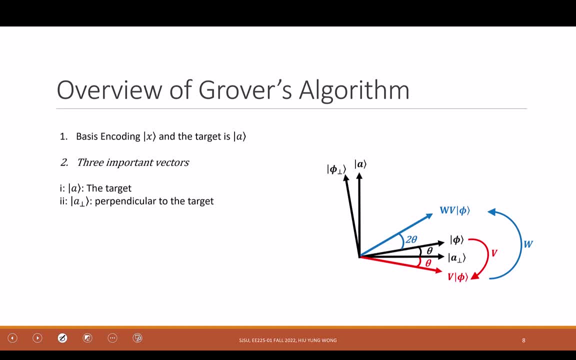 x. right, what we are searching as the basis- that's why I call it basis encoding. you need to do this encoding and you need to transfer your function into that. is that okay? just remember this, right, we are not doing the detail yet. then we have three important vectors. the first: 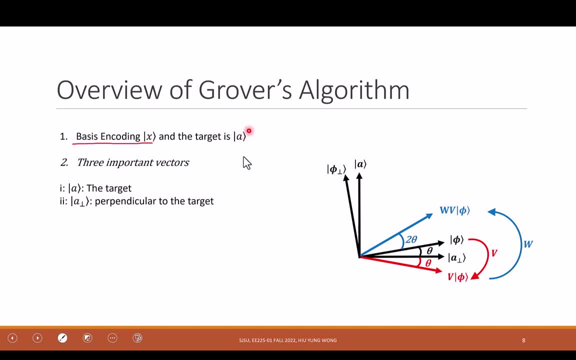 vector is the target, right, I encode it right. so a is what I want to search for. so a is the target. I draw it here: vertical 9. then there's another vector, perpendicular to a. what is that? the a is multi-dimensional, right. just now we show 5 qubit, right. 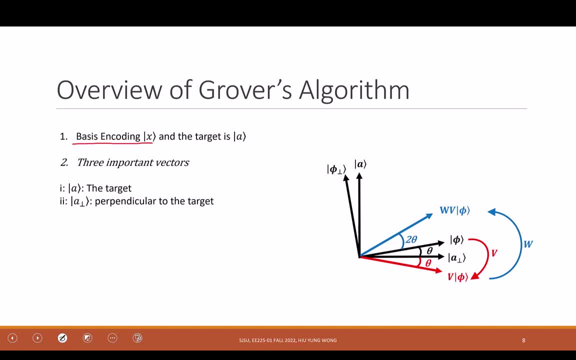 so what will be the a perpendicular b? we define it as a linear superposition. of course we know. a- maybe you can tell me what is a inner product? a perpendicular 0? why? of course yeah. so a- we define it perpendicular. we define as a linear superposition. 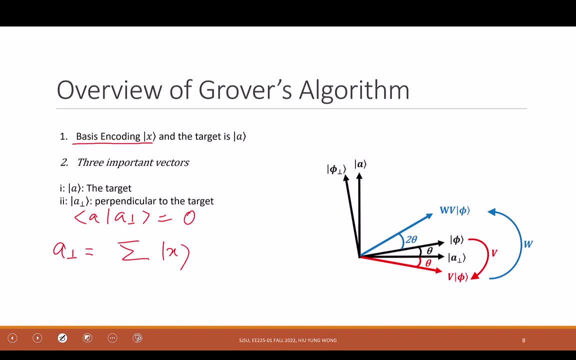 of all x, except x from 0, but x not equal to a, all the way to 2 to the power n minus 1. okay, where 2 to the power n equal to the number of entries we are going to search. I have 1024. 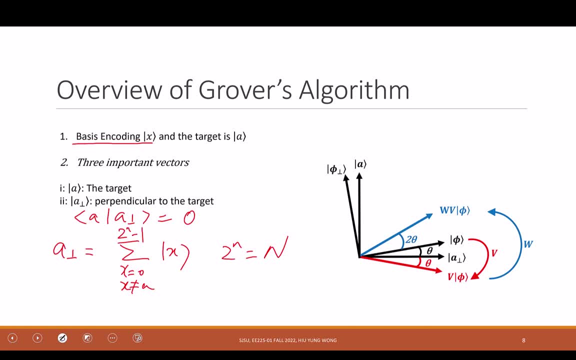 entry. I need how many qubits? if I have 124 entry, 124 student, 1024 student, how many qubits do I need for this problem? for I mean for encoding 10 right, because 2 to the power, 10 equal to this, so I only need 10 qubits. 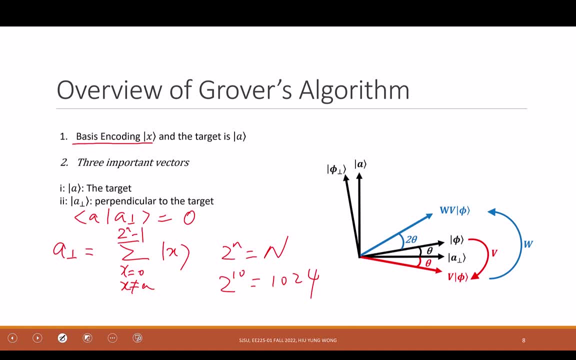 right. so I will go from x, equal to 0, all the way to 2 to power n minus 1, which is 1023, but not including a right. basically, this is 0 plus 1 all the way to a minus 1 plus a plus 1. 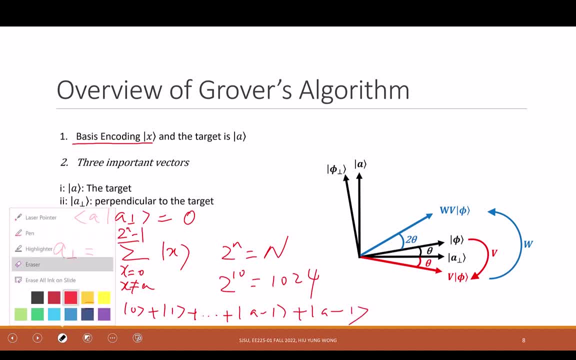 okay, I am ignoring the a right and plus all the way to 2, to the power n minus 1. okay, in this case is 1023, okay, yeah, yes, it has more than 2 dimensions, but isn't that this vector is just one vector? think about this. 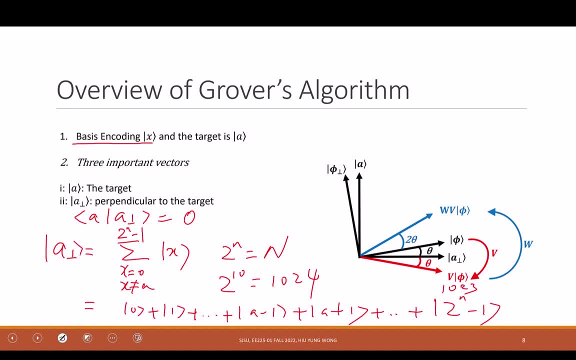 how many vector do I have here? very good, right, he is asking why I only have one vector. I am only just talking about. this vector is what I constructed to be a linear superposition of all the basis state that is perpendicular to a. that is one vector, right? 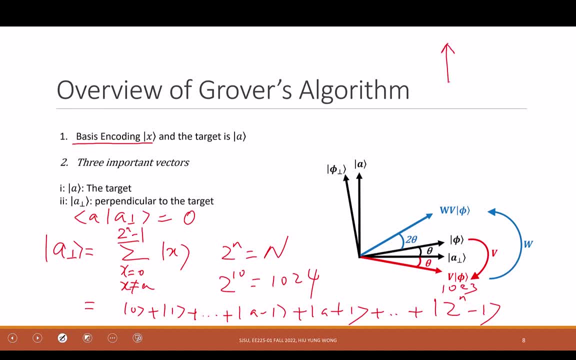 so think about this: if it is 3d, if this is a right, then this is a perpendicular. if it is 3d, do you see that right? I have one vector here, one vector here. this is the one perpendicular. so I take that plane, that is that plane. 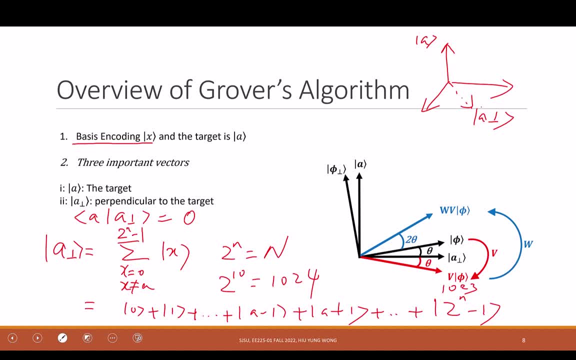 right. so if you have even 100 dimensions, it is still one vector. I can project on a 2d plane right. very good, but I need to normalize it right. this one is a little bit complicated. how many vector do I have here? 2 to the power n minus. 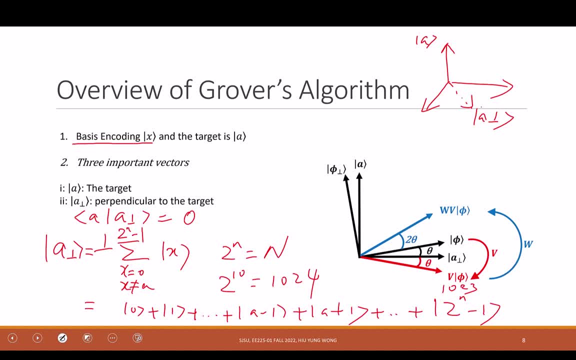 1. right, so I normalize by square root 2 to the power n minus 1. ok, so a little bit confusing still at this stage. but remember, I am just introducing an overview. we will go to the details. the point is we encode the number as the basis. 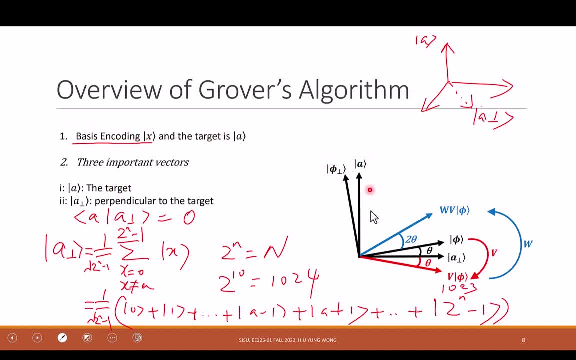 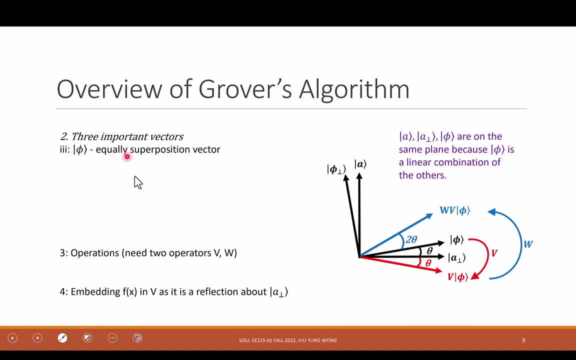 and then we have three important vector: the target a, and then we create another perpendicular to it. for some reason we call it- we will know later- a perpendicular. the last important vector is psi, which is just an equal superposition. so what is that? you should be able to tell me what is that. 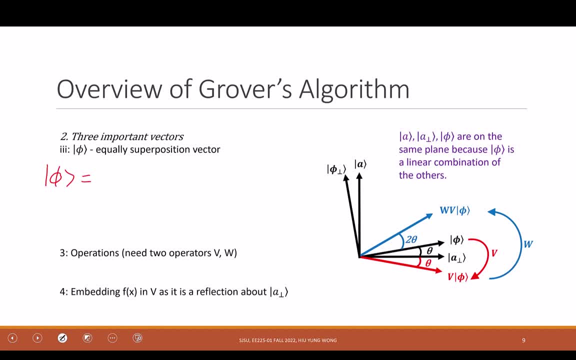 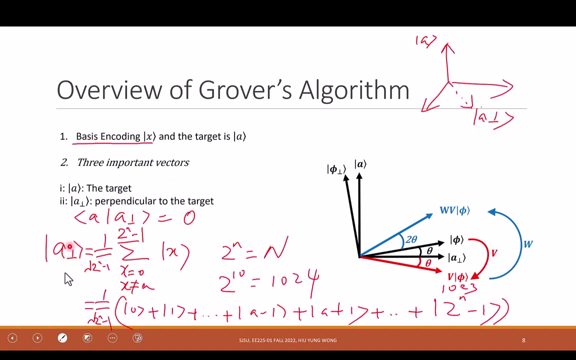 of all the basis vector summation: x equal to 0, 2 to the power n minus 1. x right, and I do normalize it: 2 to the power n divided by 2. what is the difference between this one and this one? yes, this one contain all. 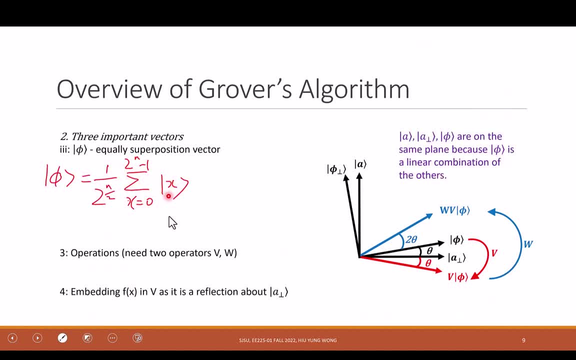 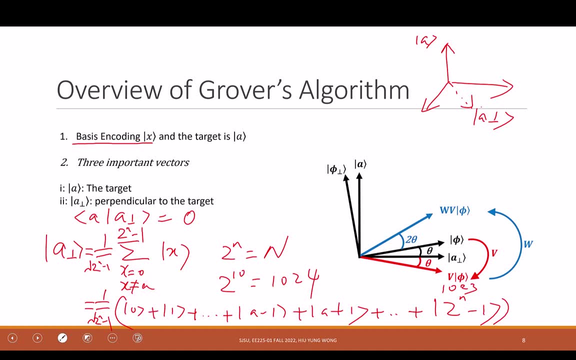 vector is a superposition of a and also other basis vector. this one we take away a. ok, so basically it is good that we drew this. this is the vector psi. it is a superposition of all the basis vector. this is 45 degree to all the angle. 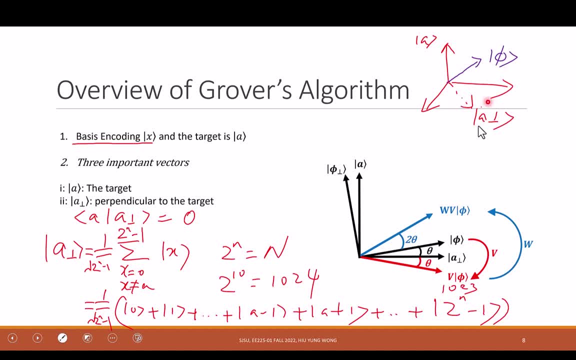 right and this is just those. this on the plane, right, but they are still on the same plane, because psi is just a linear combination of a and a perpendicular. right, because a and a perpendicular, the only difference is that one of them has a. one does not have a right and psi is. 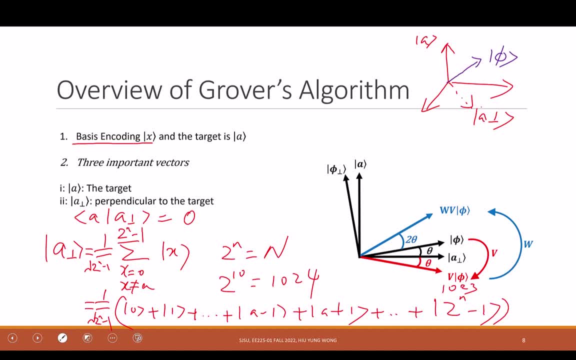 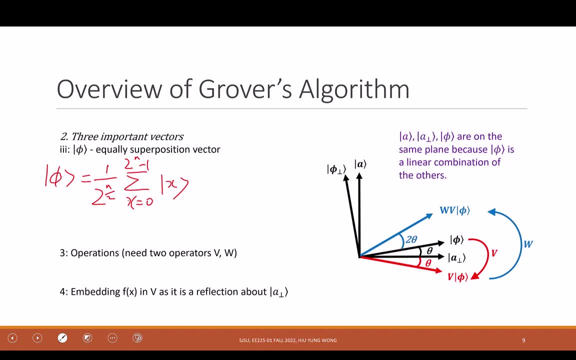 I have everything. it is still a linear combination. that is why I can draw psi on the same plane. so I am still on 2D plane. but I am rigorously correct. a is going up, a perpendicular is horizontal, and then I have psi. do you see? the psi is very close to. 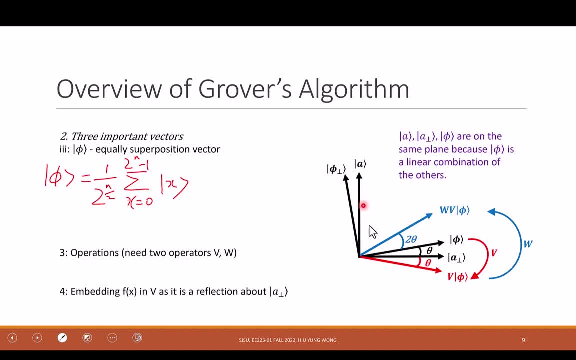 a perpendicular instead of a. why any suggestion? because almost because a psi has all the components of the basis state except, I mean, has everything right, and a perpendicular also have the component of everything except a. now, if you have a dimension of one trillion, the a component is very. 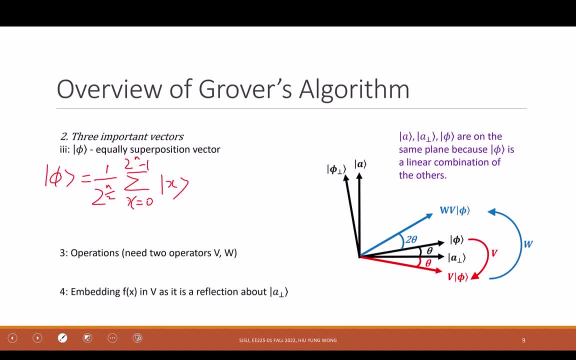 tiny, make sense, and that is why psi is very close to a perpendicular. okay then, what do we do? we will invent an algorithm which is Gouffre's algorithm. it has two operators, one is v, one is w. it first will flip psi about a perpendicular. 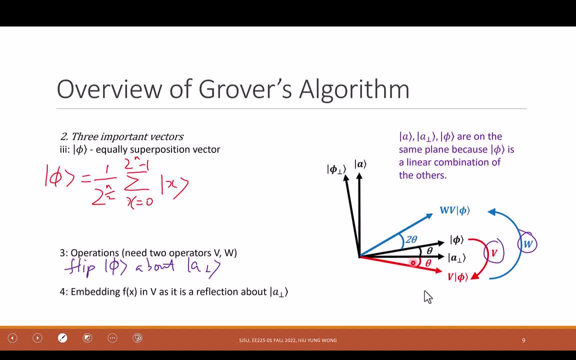 okay, then I get this one. the second step is: this is v, w is to flip the vector, any resulting vector about psi, like here. and then what do you do? repeat again, flip again, repeat again, flip again, repeat again, flip again, and then the final vector is a. it aligns. 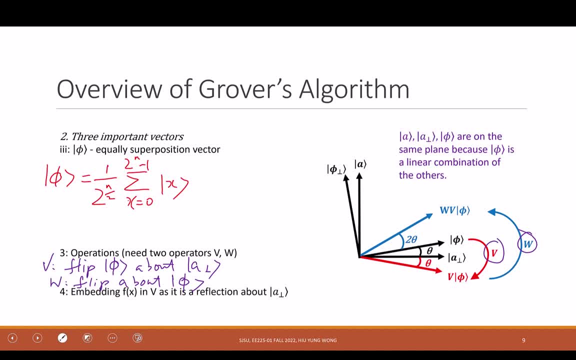 with a. that is the idea of Gouffre's algorithm. okay, and this operation only take you square root n time. you only to need to do it square root n time when I flip about. some of you are trying to pointing right. flip about v you actually. 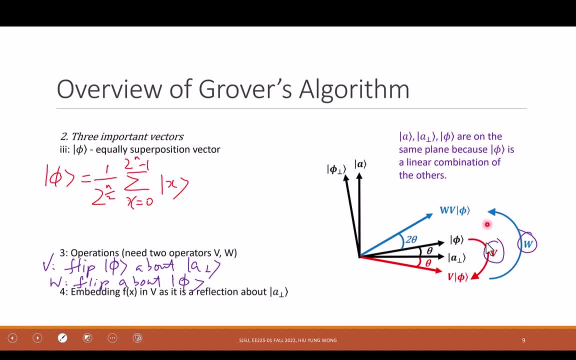 rotate it by two theta, then you go up. you rotate it by two, four theta, you go down again. you rotate it by no. here it will be six theta, right, because about eight per centimeter. but if you say this, yeah, and then you go up again, so you, you just go much faster. 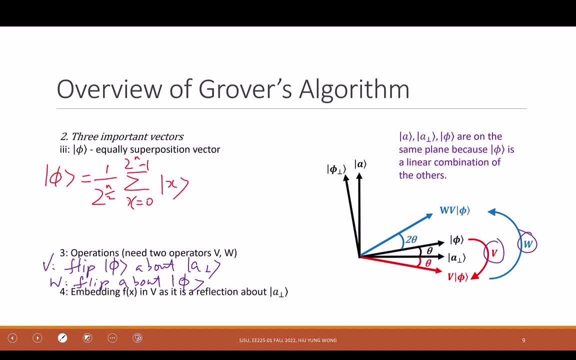 like every time you go up. that's why you give you the square root. but the point is, you see that this algorithm eventually will bring your solution, psi, which is a superposition to only have the a component, and you measure it. then you know what is a. 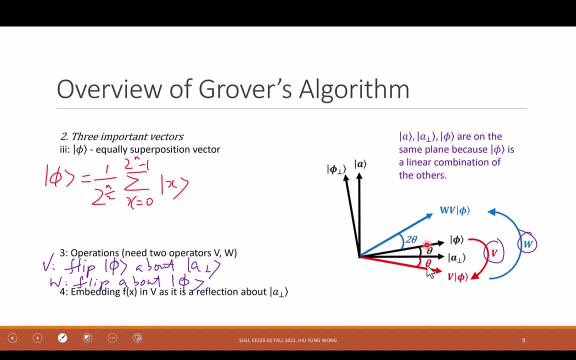 at the beginning you only have psi right. you measure it, you get all the probability of getting zero, one, two, three, four, all the way to two n minus one. but after all this flipping it's basically just a. you measure it, you only get a. if you don't do it well, you will. 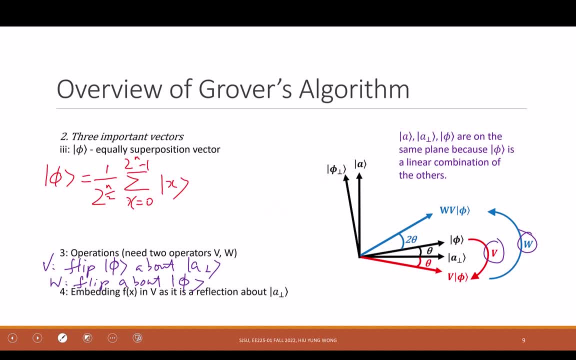 pass a. but here you will do something. be careful not let you pass a and also think about if it's very close to a. you have a very large chance. you are at a already. maybe you can just verify. right, you say, just do a lot of square root algorithm and then identify. 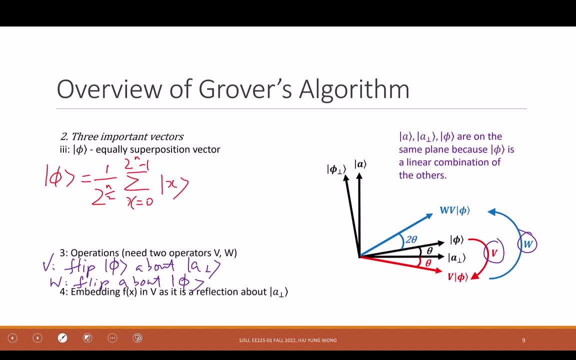 maybe you are the student i'm looking for. maybe i get it wrong. actually i got another one. you say no, then okay, do one more time again. square root is useful, right i? maybe next time i get you, yeah, but of course there are many details i don't know, right. but 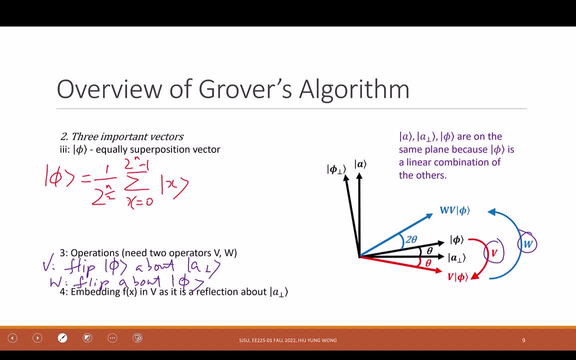 that is the idea, right. so this is rotates two theta and this is rotates four theta. right, this is clockwise, this is counter clockwise. right now, actually, when i do this flipping, what do you think? i still have not thought about the f? x, right the function. the oracle must embed something, right? so 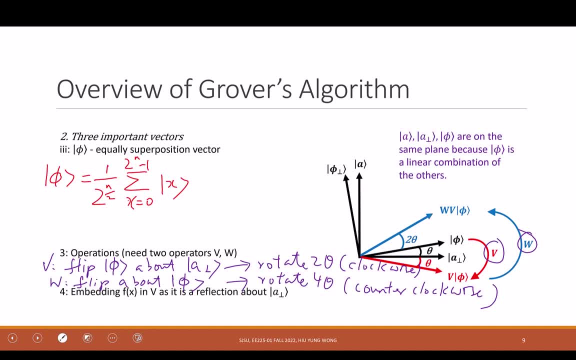 where should i embed this f of a? the vector cannot embed f of a. it must be the operator right. which operator makes sense to embed the f of a? do you think it's v or w? yeah, it is v. very good, it must be in v, because v is about. 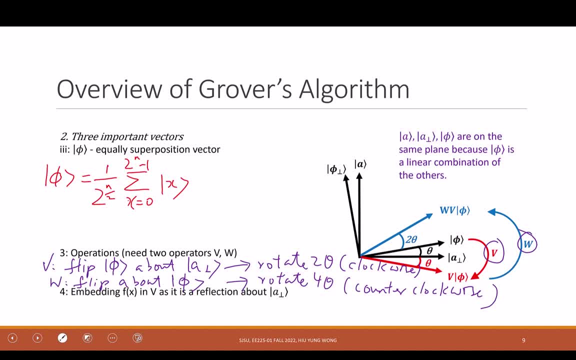 rotating, flipping a about a perpendicular? yeah, it doesn't have a. it means that it contains information of a right. it has everything but a. it means it has the information of a. you know what a is, so we are going to use this v to do the f of a calculation. 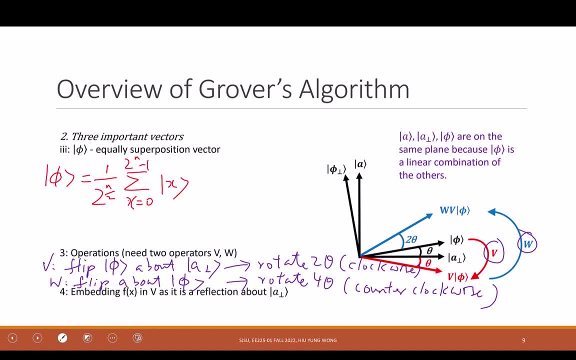 which will be a phase oracle. okay, we will see that later, but i hope that you can appreciate, uh, overall, what we are trying to do here. is that? okay, what happened to what w is still useful. it's going to use for flipping. but i want to contain the info where. 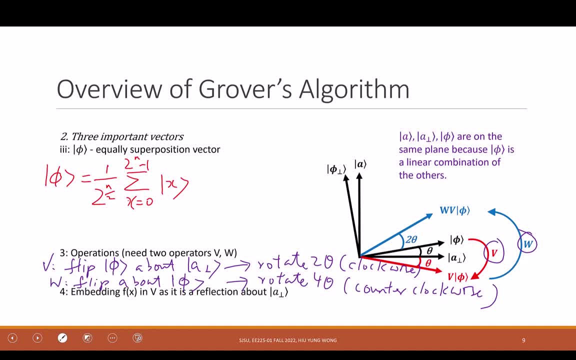 can i find the information of f of a? where should i embed the f of x information into? i will embed into v right, because it's rotating about a perpendicular, right. then it must be there because the rotation of w has nothing to be to do with a perpendicular, it is. 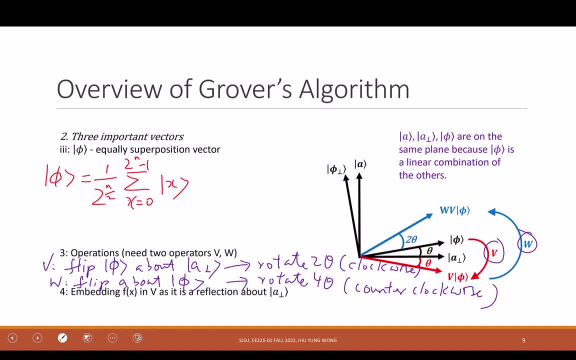 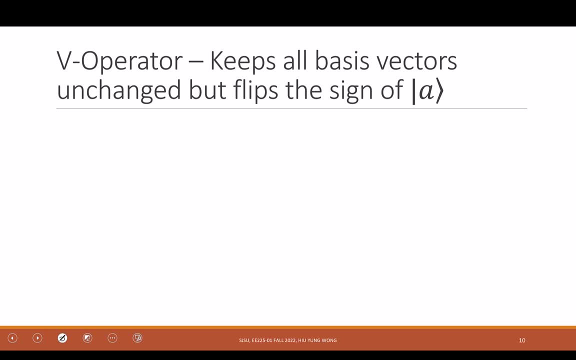 above phi right. very good, so let's start doing one by one right. how do we implement the v operator? so we are going to define? this is like the genius, they find it out. all we need to do is just to verify it is correct. we say we are going to do a v. 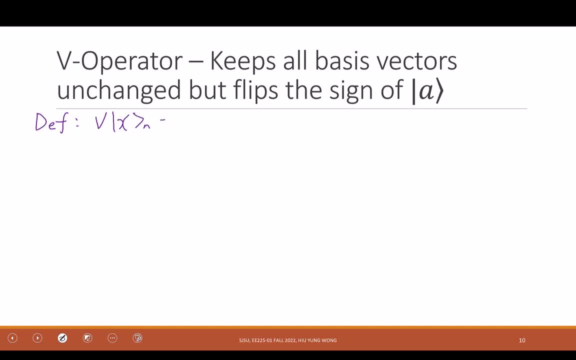 apply to the basis state and is equal to negative one f of x, xn. so this is a phase oracle. okay, so we are going to implement v using a phase oracle. how to do it is another thing. assume we can do it, okay. so what does it mean it? 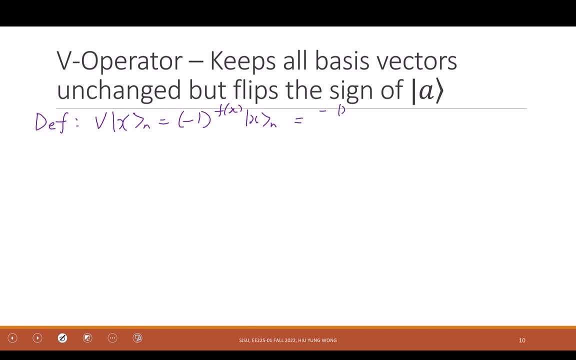 means this is equal to negative xn. if f of x equals to a, because it give you one right, is equal to x. if f of x not equal to a, because it give you zero right. basically it is saying that if x equal to a, i will get negative. 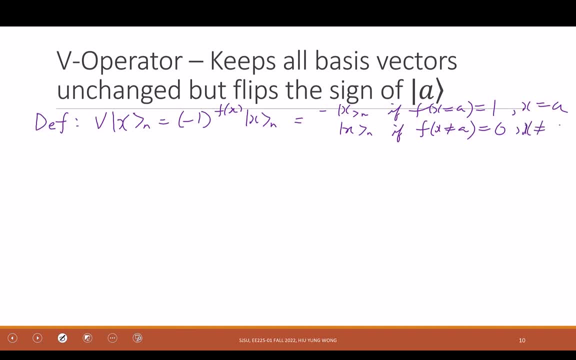 if x is not a, i will get positive one right, because what problem? what we solving? we are trying to find out where is which is the record i'm searching, right, and when it is a the one i'm searching, you should give me one right. so, as a result, 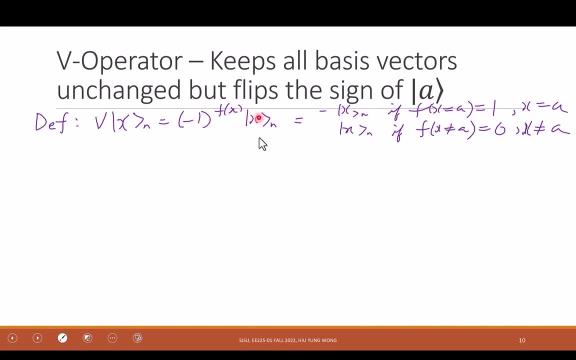 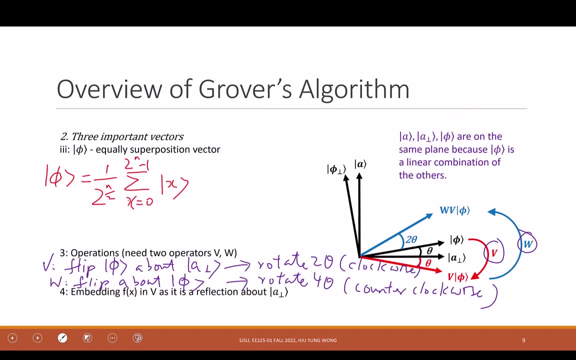 negative one to the power. f of x needs to be this one right. if it's not what i'm searching, then f of x is zero, then this is positive. negative one to the power, zero is one right. so this that's it. so this is the oracle, or? 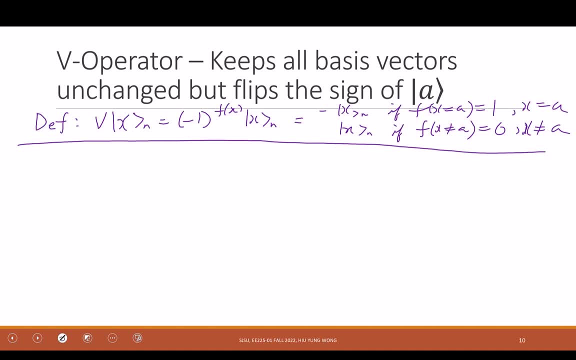 the v option that we are going to do, but i need to prove to you that it does flip, right. uh, so now let's check the property. right, this is done already. right, you come up with this. so let's see for general vector: right, for any vector. 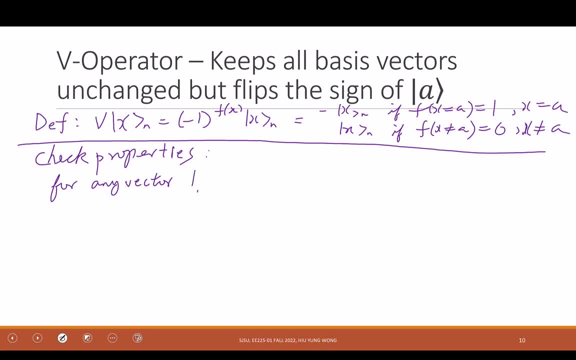 for any vector. i can always, always represent it as: beta equals to summation, x equal to zero, to the power n minus one, beta, x, x. do you understand this equation? right? it's just a linear combination of all the basis states, right? it's basically saying: okay, any vector, any. 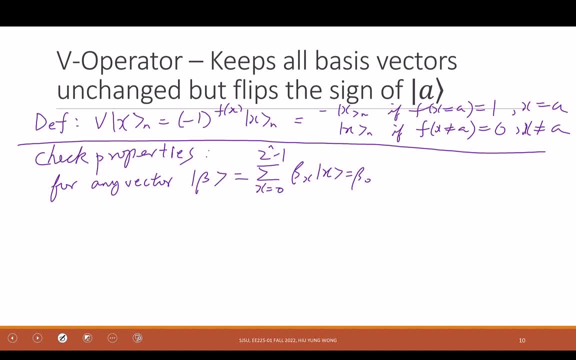 n-dimensional vector. it is beta zero times zero state, beta one times one state, all the way to beta two, n minus one times two, to the power: n minus one state. that's it. that's, that's a general vector. right, let's see what happened. does it really do the rotation we want? 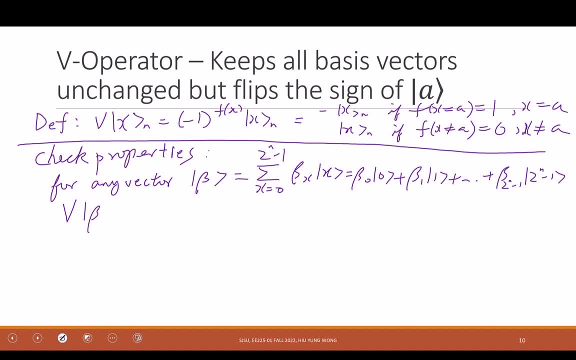 if i apply the v to beta, okay, by the distribution loop right, this is equals to the beta: zero negative, negative one to the power f of zero, correct, right? this is the rule: plus beta one negative one to the power of f of one, plus beta a negative one to the power. 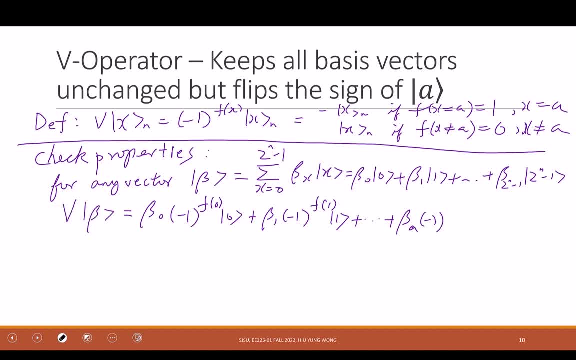 beta f of a, a right because a is at the one of the vector. also, i don't write the rest. all of them are zero when they are not equal to a. so these are positive, except that when it is a, this is negative because f of a equal. 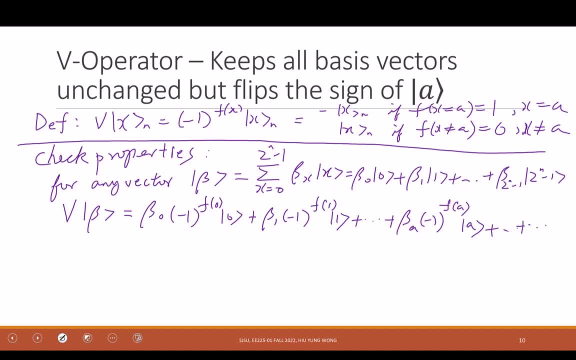 to one, so negative. one to the power. one is negative, so this one: give me beta zero, zero. beta one, one negative one. i mean maybe i will just write negative beta a, a, and then the rest are still plus beta two n minus one. two n minus one.